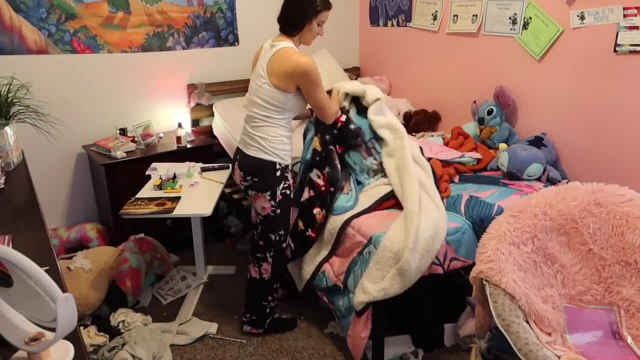 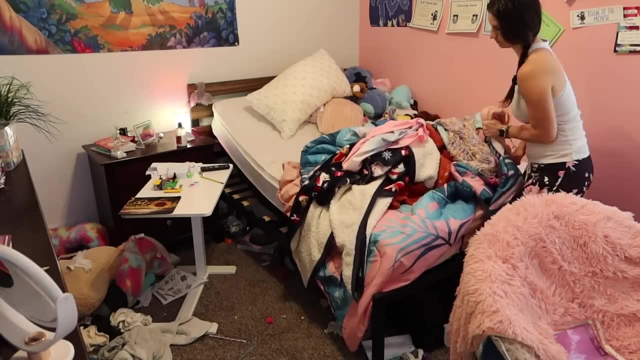 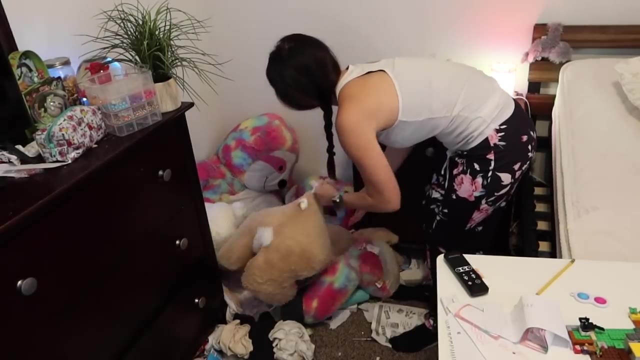 that, as you can tell, it messed up my voice and I tried to put off this voiceover for literally four days, hoping that my voice would go back to normal, but unfortunately it is still bad. It is so much better than what it was, So I'm sorry You guys are going to have to listen to. 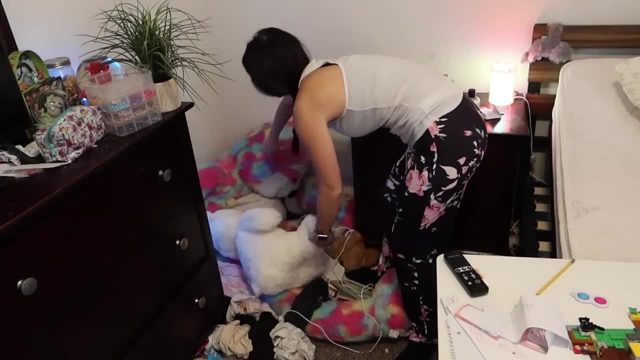 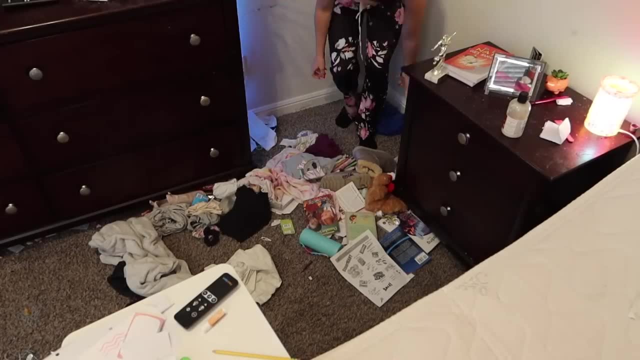 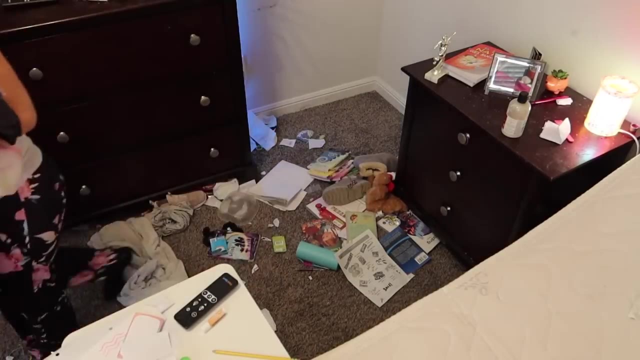 me sounding kind of funny, but that is why I unfortunately did catch that stomach bug. Thankfully it was only 24 hours, but oh my gosh, it was awful. But today's video is a super motivating one. The before and after transformation is amazing. 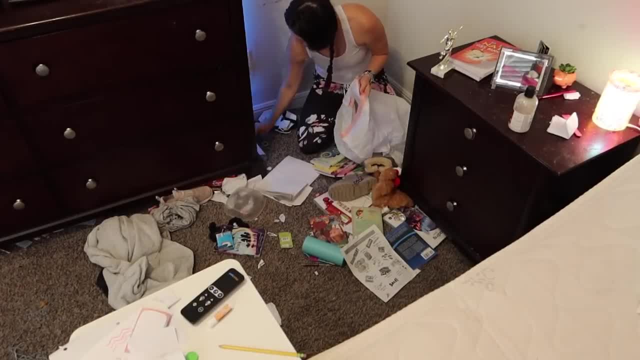 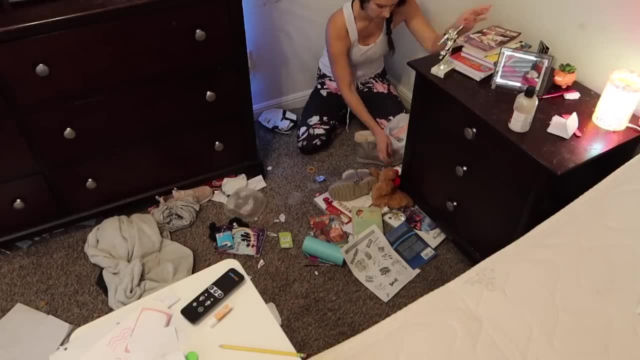 I know you guys love this video because of that. Like every time I clean her room, you guys enjoy it, So I hope y'all still enjoy it, Even though you have to listen to me sounding crazy. but first things first. we are going to be starting off by getting all the trash. 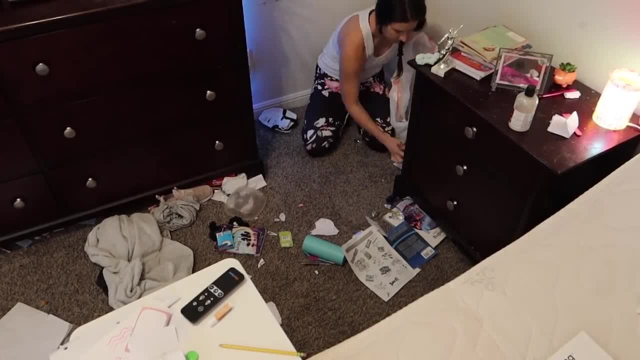 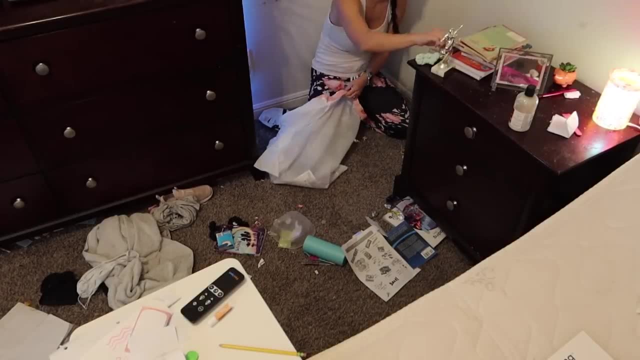 off of the floors, As you saw, I pulled off the bedding. I want it to wash it, get this room sanitized, wipe everything down. I'm going to be doing a lot of cleaning, So I'm going to be really well just to get all the germs out of here Fingers crossed. No one else is going to. catch it. so far Only the three of us have got it. So three of the other kiddos have not caught it, which they just got over a stomach bug like a month ago. So I'm hoping you know that was the only one that they were going to get, but I don't know. We'll see. 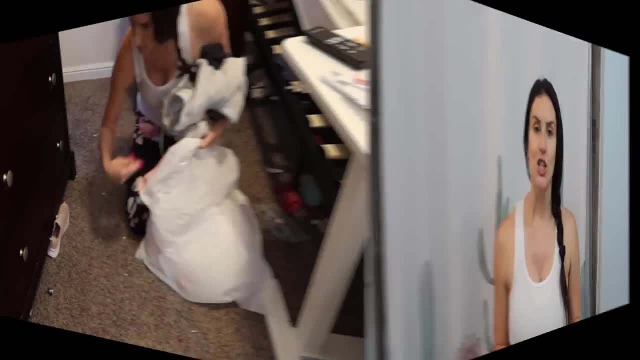 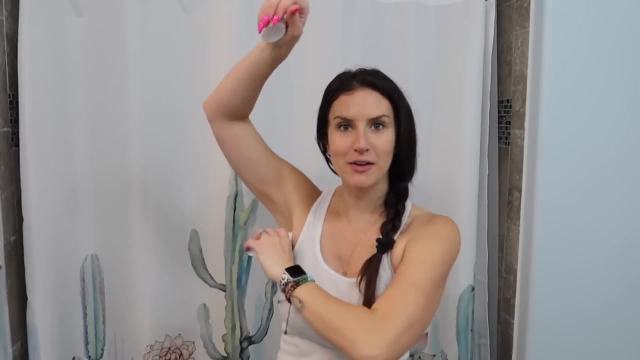 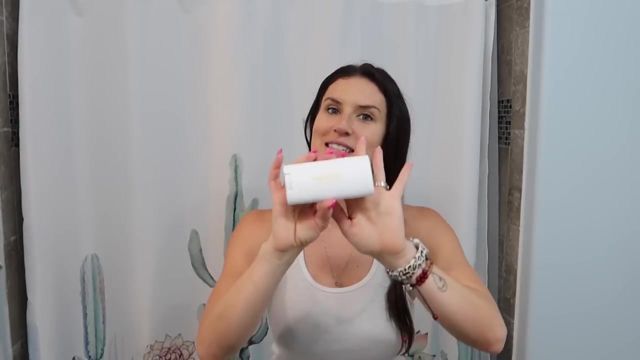 Just a quick break from today's cleaning motivation to freshen up a bit. Y'all know you get hot and stinky when you are cleaning, which is why I'm really excited to announce today's video sponsor, which is Native. I have been using aluminum-free deodorants for quite some time now. 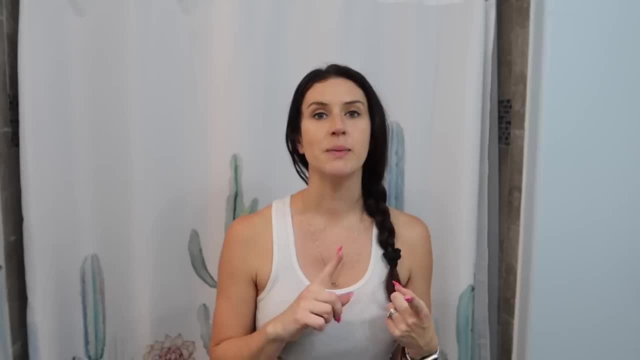 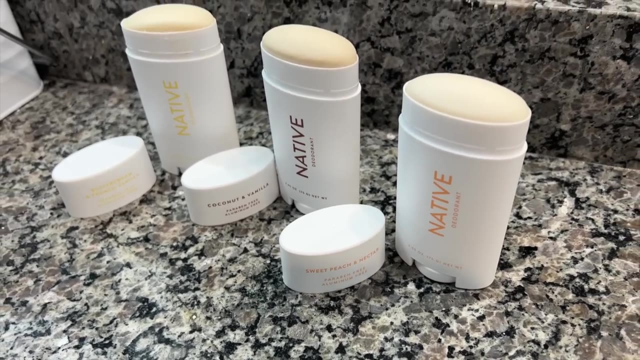 and Native has always been my go-to one, not only because they're aluminum-free, but they're also paraben-free, cruelty-free And vegan. A huge reason why I always gravitate to Native is because of their scents. They smell. 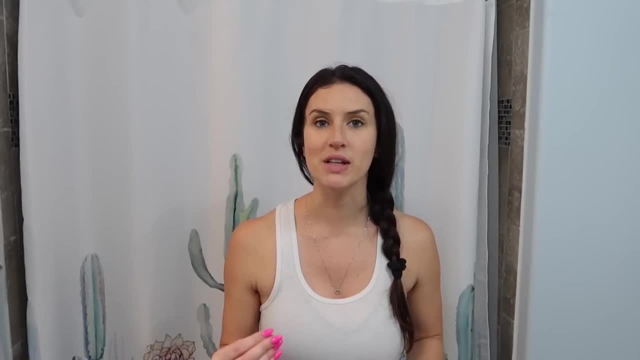 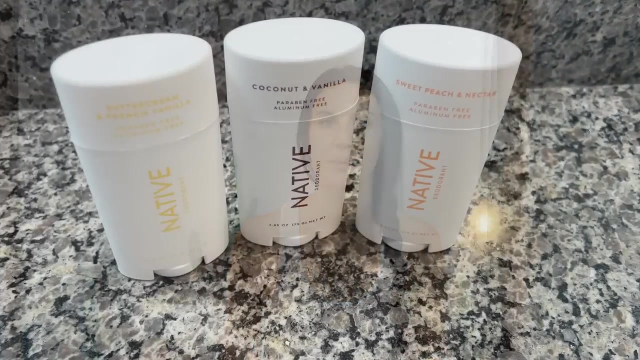 amazing. And not only that, but they last you a really long time- up to 72 hours of protection, So you don't have to keep reapplying your deodorant, because you stay feeling fresh all day long. And whenever you apply your deodorant you are not sticky and it's dry immediately. The three scents: 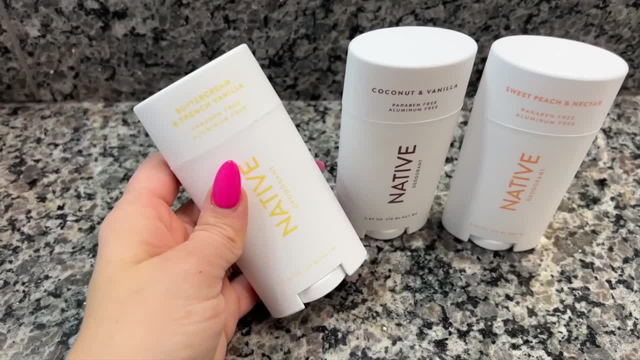 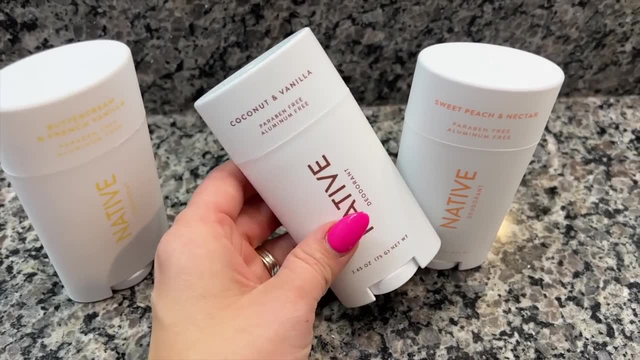 I went with was buttercream and French vanilla- my all-time favorite, You guys, it smells just like a vanilla candle. I am obsessed. The coconut vanilla, which is another amazing scent- It's definitely my second favorite. And then I have the sweet peach and nectar. 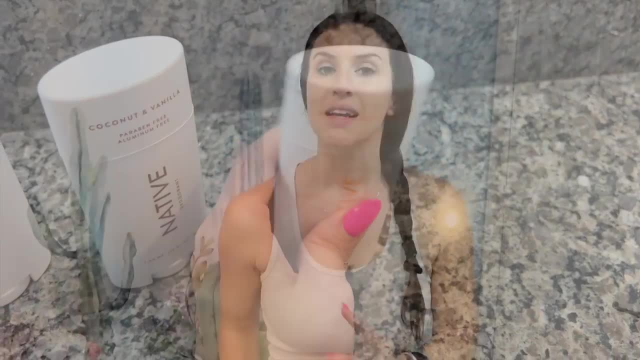 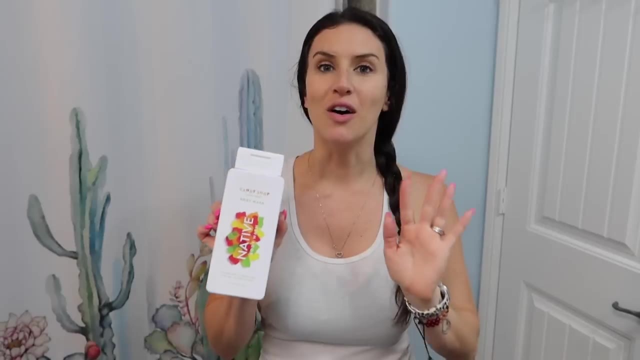 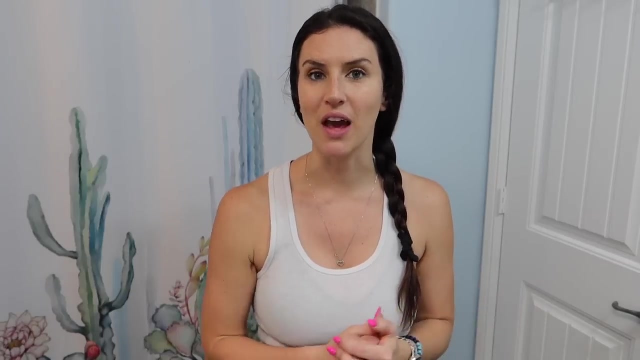 which smells so good. It smells just like peaches. Native also has body washes and lotion and they just came out with their new candy shop collection. They all seriously smell phenomenal. This is the gummy bear scent. It's so fruity and delicious I had to go in stores to smell all the. 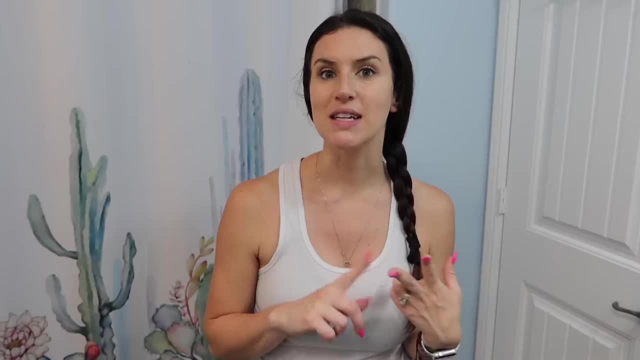 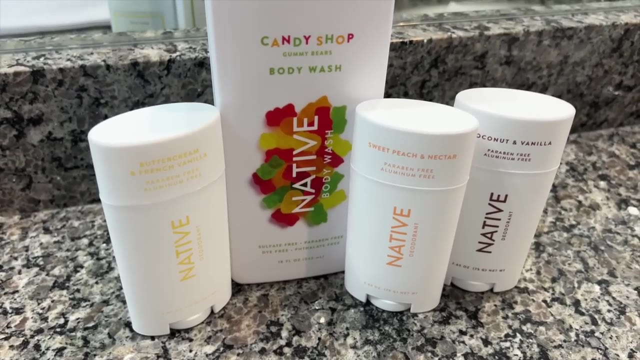 scents, but they did come out with sweet cinnamon hearts, sour berry belts and strawberry vanilla taffy, which all smell phenomenal. And make sure you guys don't miss out on the awesome deal they are offering my subscribers just by heading down to the description using my link and my discount. 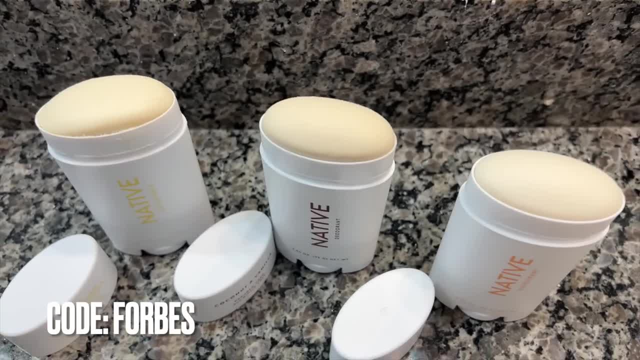 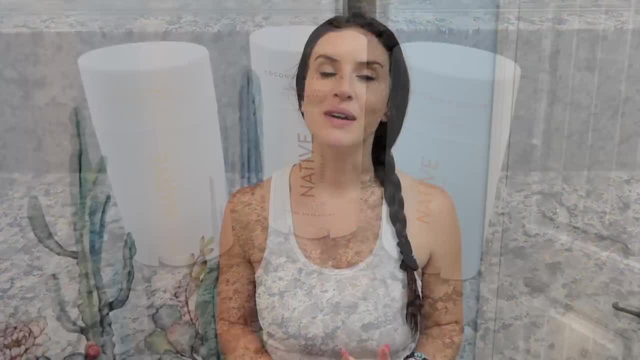 code, which is Forbes, to get 20% off your first purchase at Native. This offer is available site wide, but only for a limited time. So stock up and save, But once again, thank you so much, Native, for sponsoring today's video. but let's go ahead and jump right back into all of this cleaning. 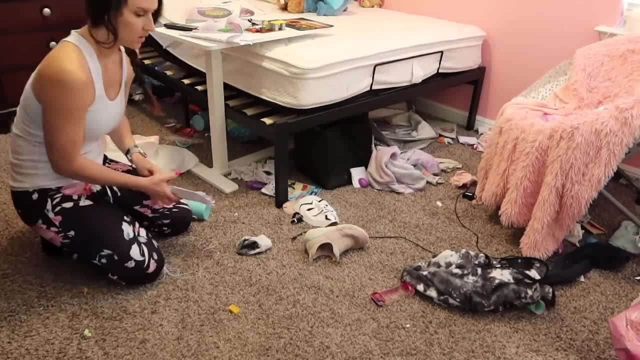 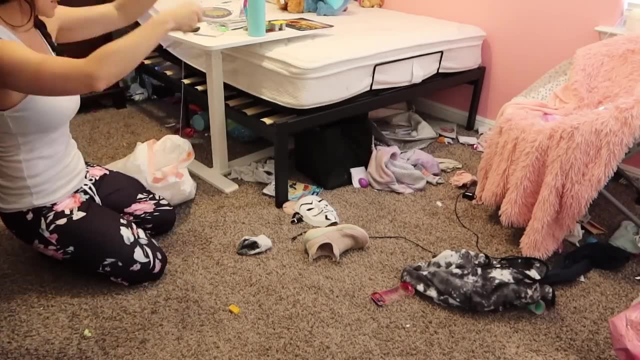 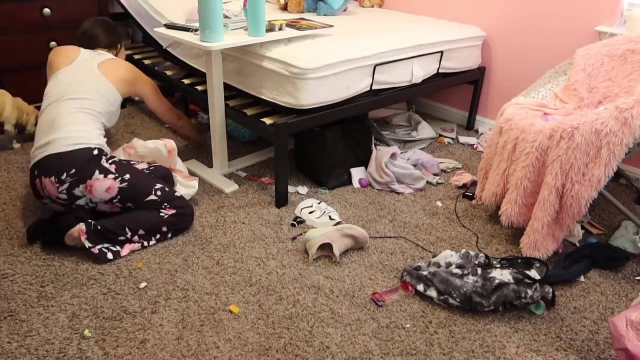 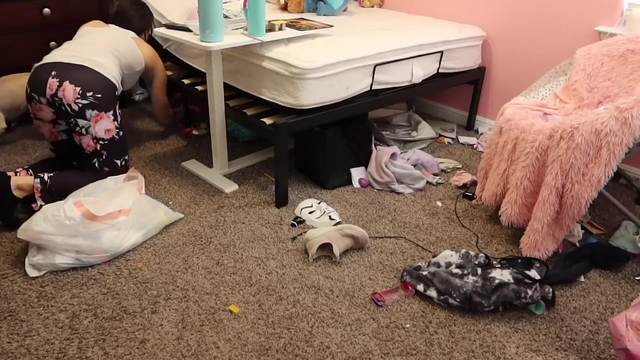 motivation. So how was y'all's weekend? Let me know if you guys did anything fun. We finally had our garage sale. I have been decluttering the house for quite some time preparing for it, And let me tell you the turnout was amazing. 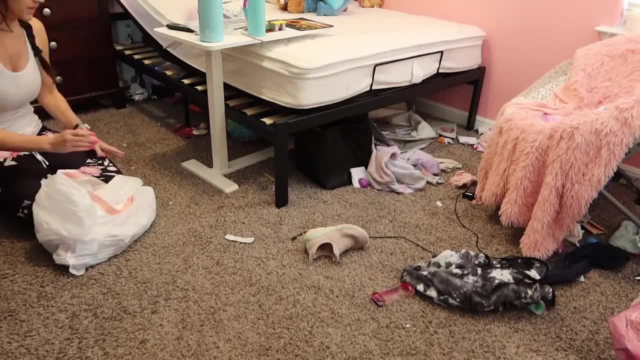 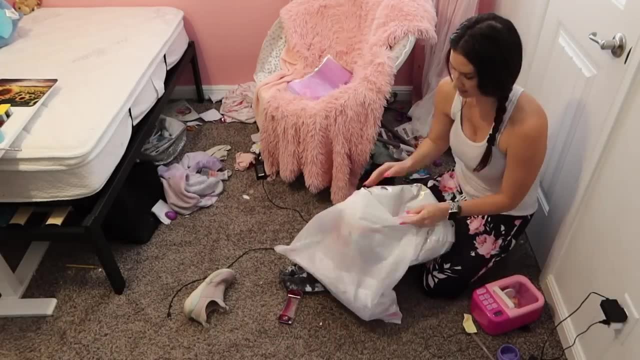 So much stuff. almost every single thing that we put out there we sold and we had some big ticket items that I was kind of worried wouldn't sell, because I feel like garage sales it's a little hit or miss on the bigger items if they're you know if anyone's going to want to buy them. 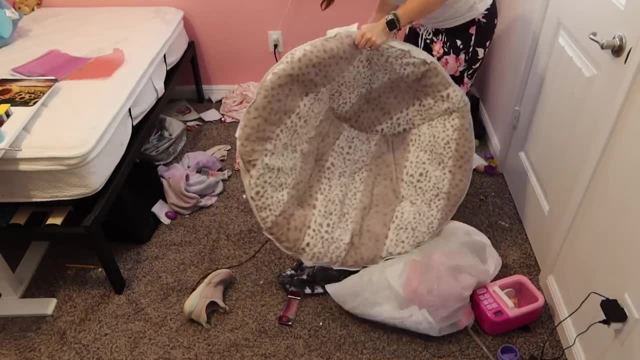 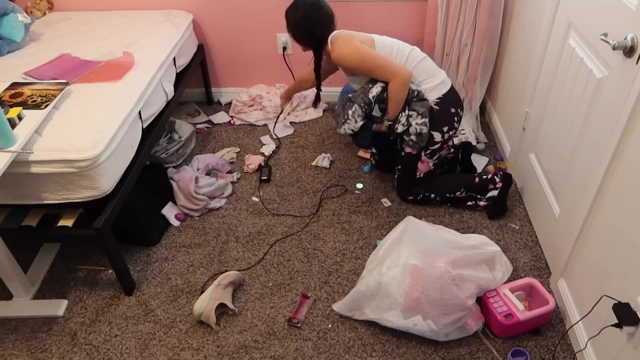 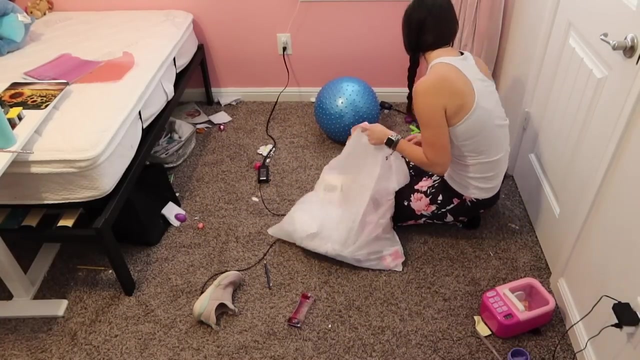 but I was able to sell our old dining room table. We sold my old rims for my car and tons of clothes and old decor. Oh my gosh, It feels so good to have all that clutter out of the house. We actually cleaned the garage out the day before as well, because it was so bad in there. 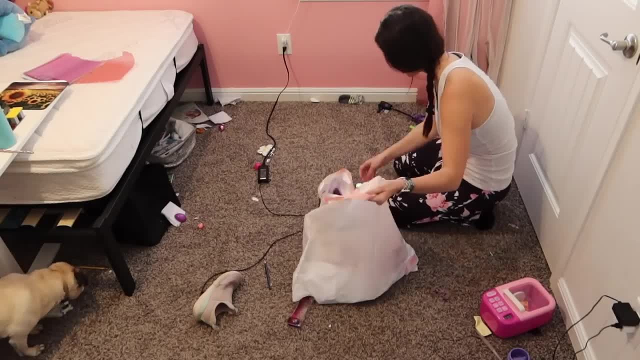 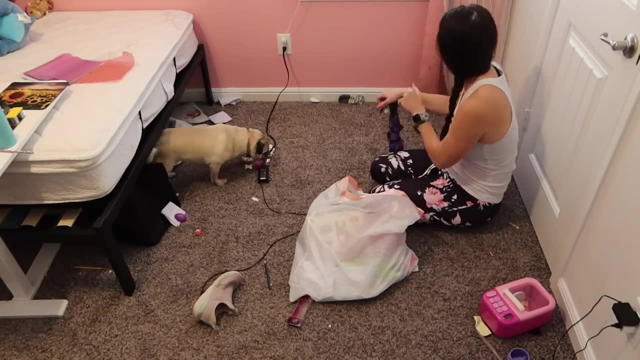 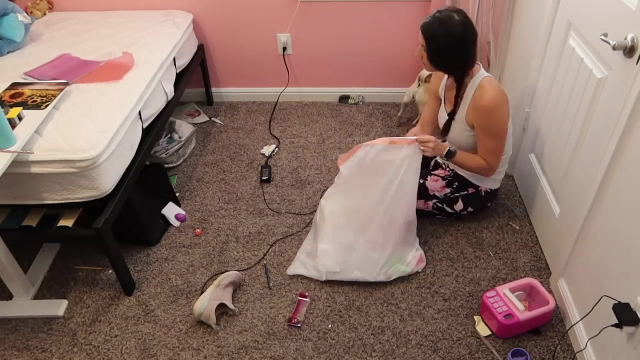 We didn't want to have our garage opened up and like people come by and it just looked a hot mess. So me and my husband cleaned it. I'll definitely have to show you guys the update on what the garage looks like, because it's seriously night and day Like if you guys follow me on my vlogging. 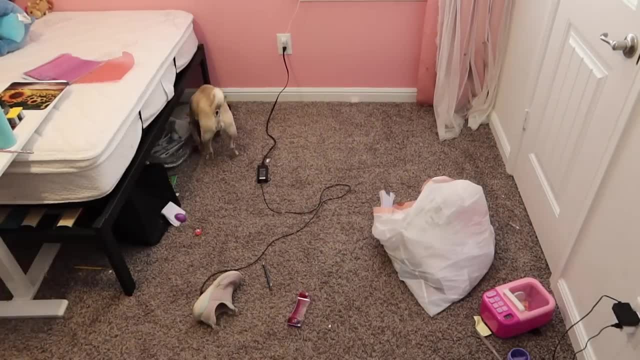 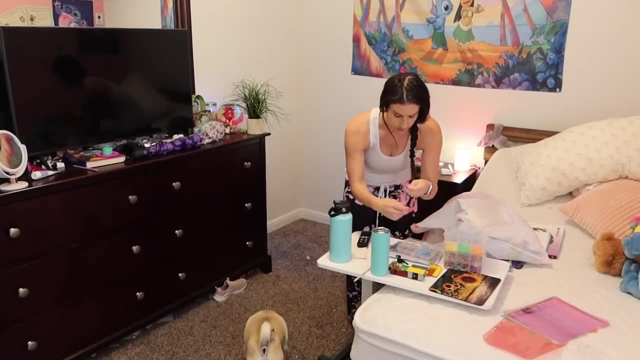 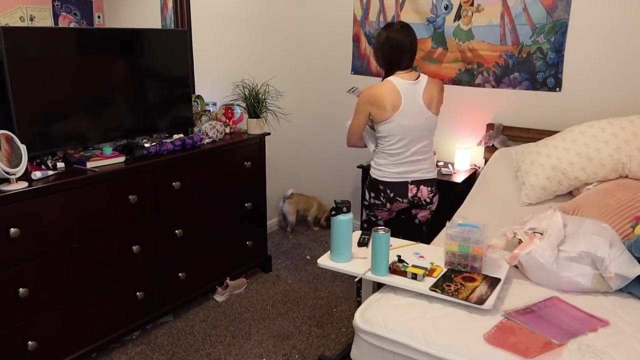 channel. then you saw it recently And we literally had a pile of bikes and we just had things stacked On top of each other And now it is completely clutter free. I mean it feels amazing, So I'm really happy we got all of that done. We really made a big dent in our storage unit. We're hoping. 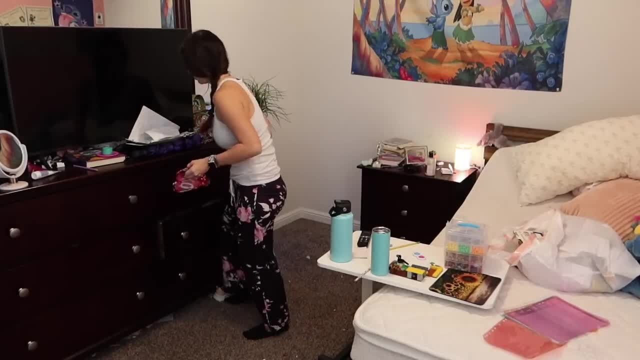 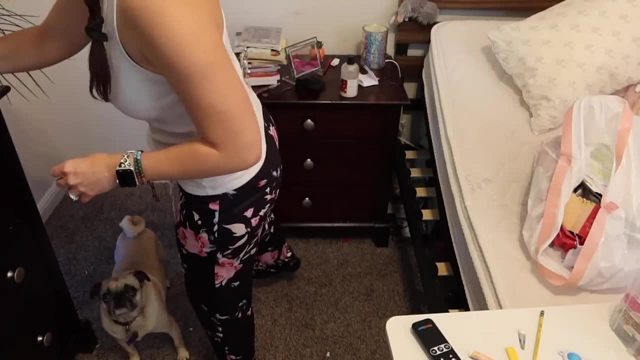 to get rid of that, but it just feels really good. So I definitely recommend, if you guys are trying to get rid of some clutter, do a garage sale. It just feels so good to get rid of the clutter and make a little money at the same time. Definitely recommend it. 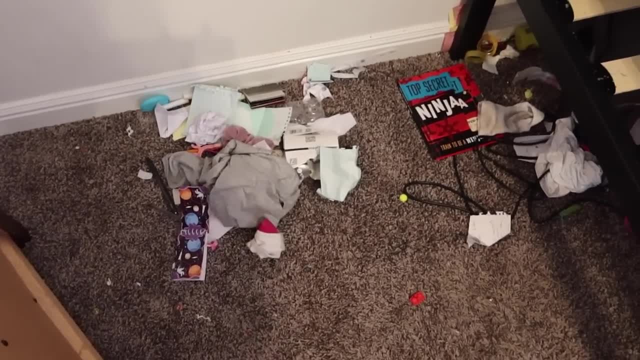 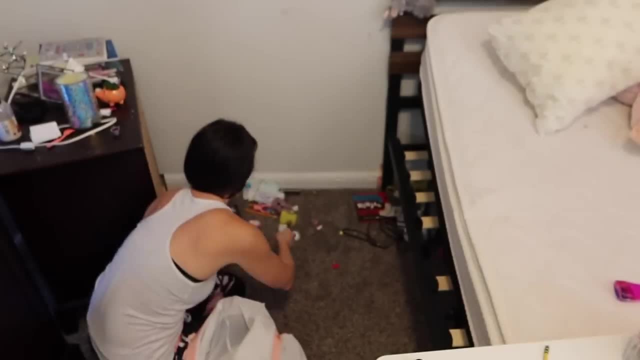 We got lucky and our whole neighborhood was like putting on the garage sales. So we knew there was going to be a big turnout of a lot of people you know coming through there because there were so many garage sales going on. So that worked out so good. We're also getting super. 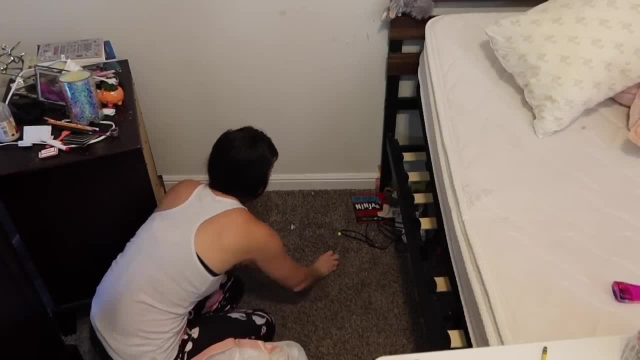 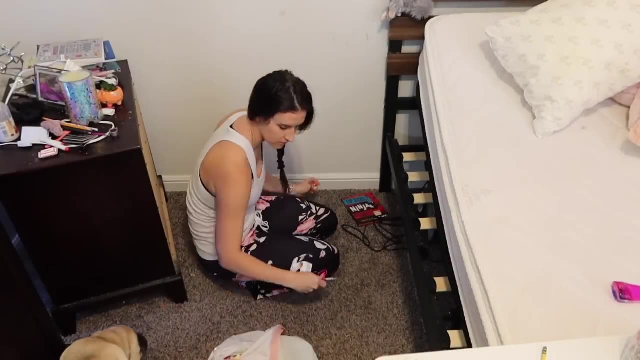 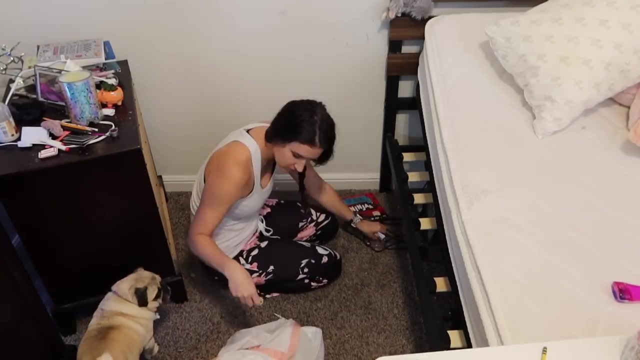 excited. Our neighborhood pool is opening up tomorrow, May 1st, So we are super excited about that as well. The kids cannot wait to go swimming and just be out and about again, because this way winter felt so long and we were sick so much. So we are ready for all the vitamin D and the 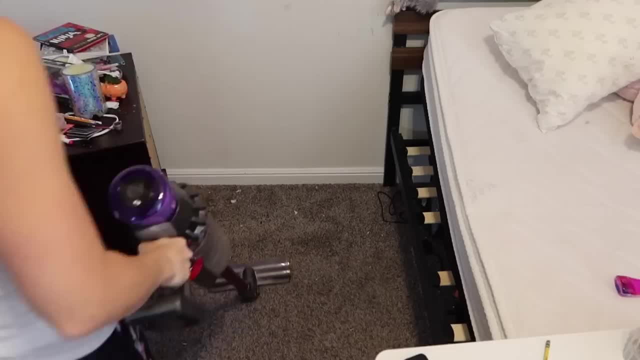 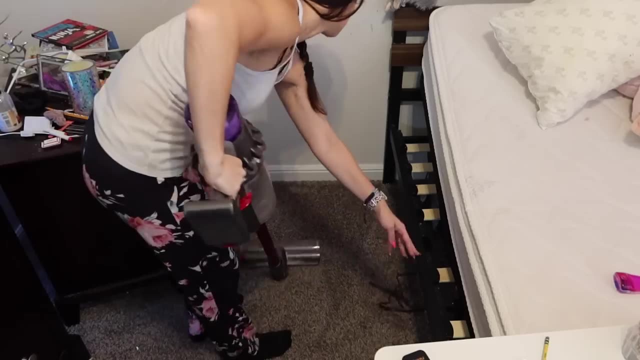 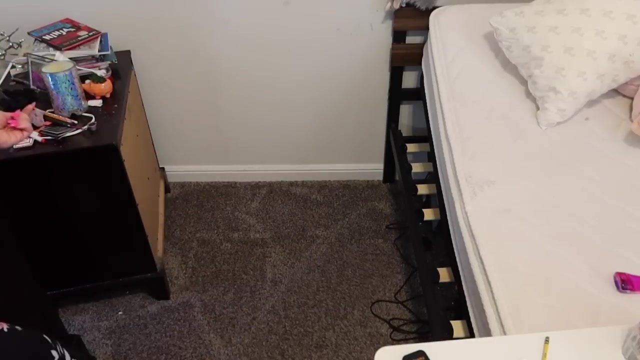 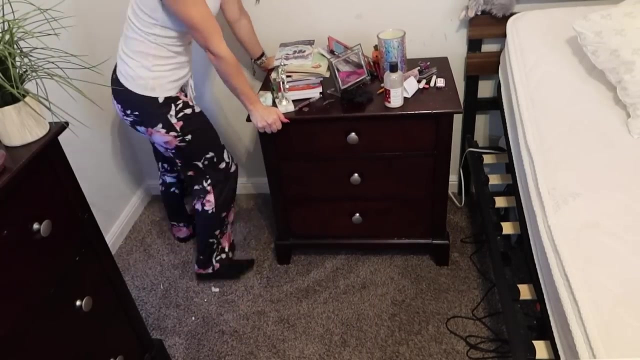 sunshine and no more sickness. I really wanted to make a point to move Adrian's furniture and clean underneath of it, because I knew it was really bad. So not only do I move the nightstand, but I'm also going to be moving the dresser and cleaning underneath of that. And oh my goodness. 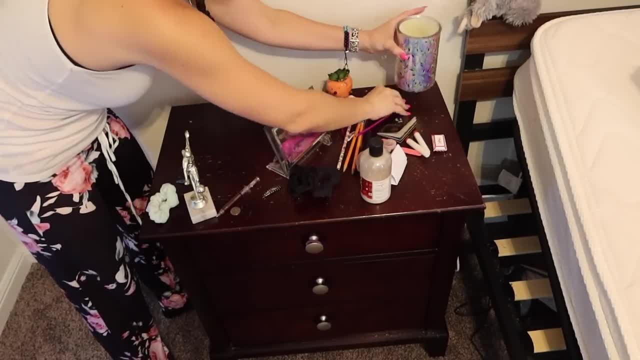 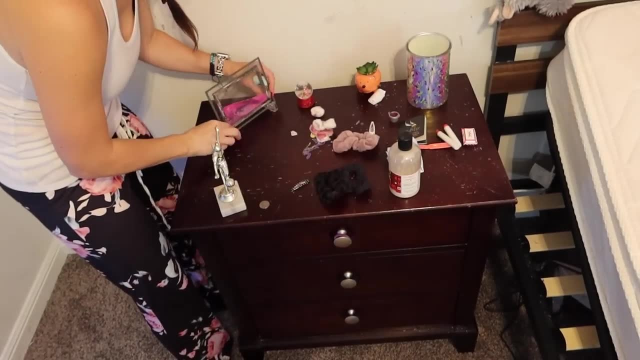 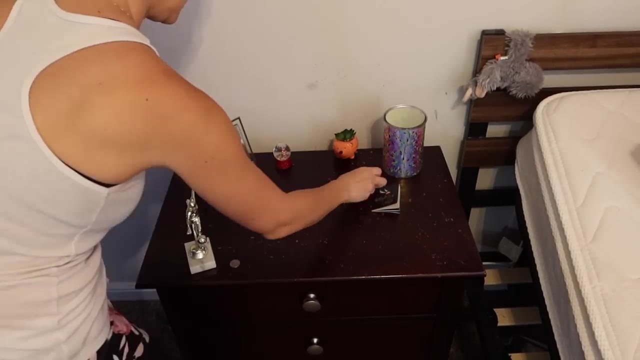 you guys. the top of her nightstand was covered in wax melt. My sister sells scentsy and she gave her her own little you know scentsy warmer. But unfortunately she was making such a mess, not only on the nightstand but you can see it's like splattered on the wall. So I told her no. 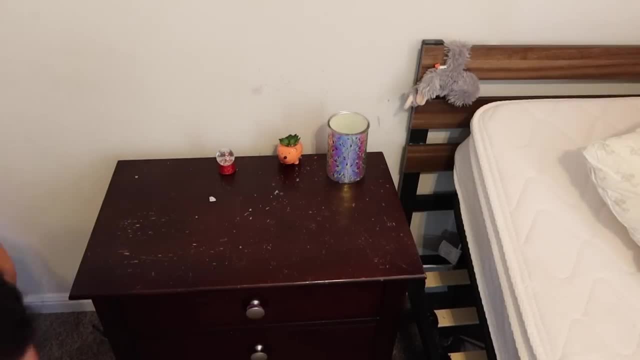 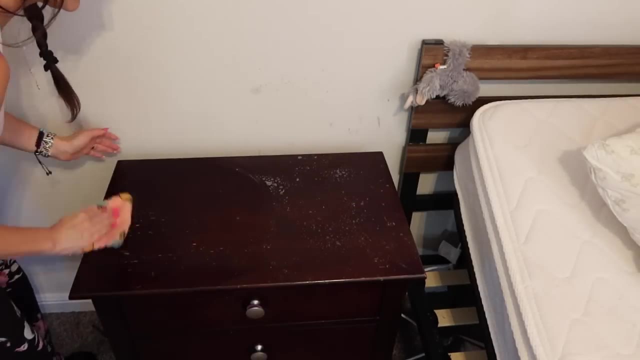 more wax melt in here. I ended up taking it out of her room, but she begged for it to come back into her room, So I told her: no more wax melt in here. I ended up taking it out of her room, but she's not going to put any wax in it. She uses it as a nightlight too, So I told her for. 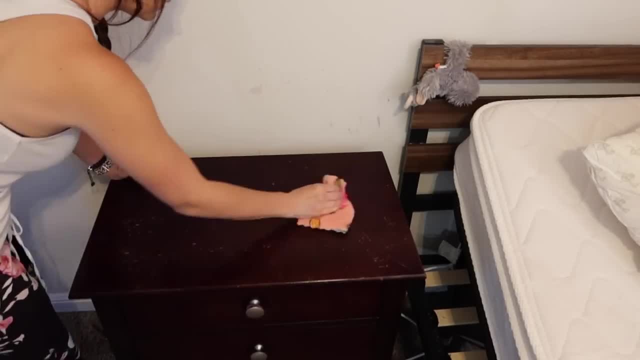 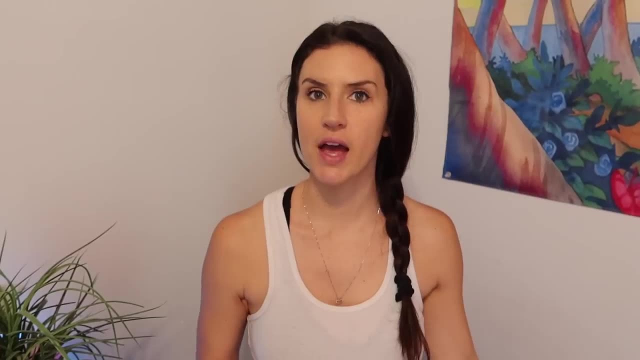 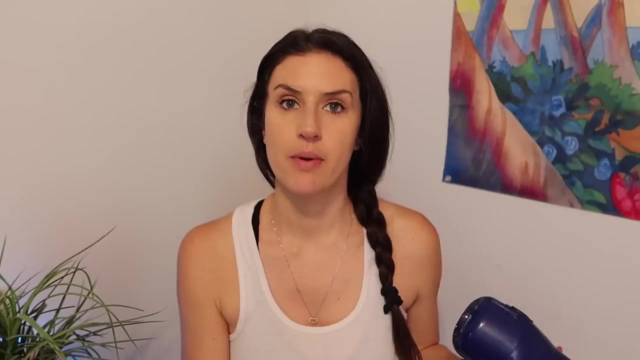 now she can use it until we get her a proper nightlight. Adrian has wax all over her nightstand and I've heard the hack where you just use a blow dryer and some paper towels and you like, put the paper towel on top of the wax and you heat it up with a blow dryer and you should be able to wipe. 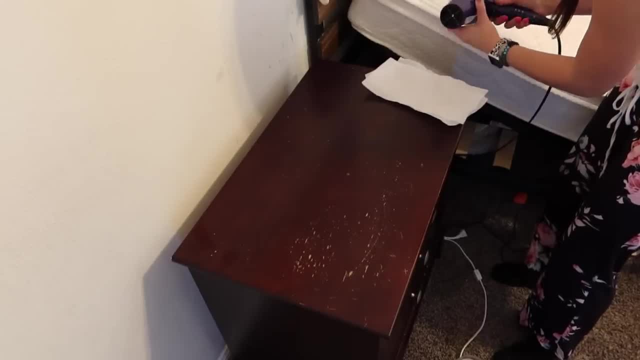 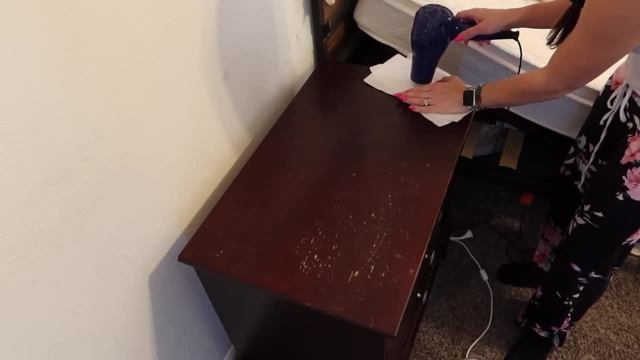 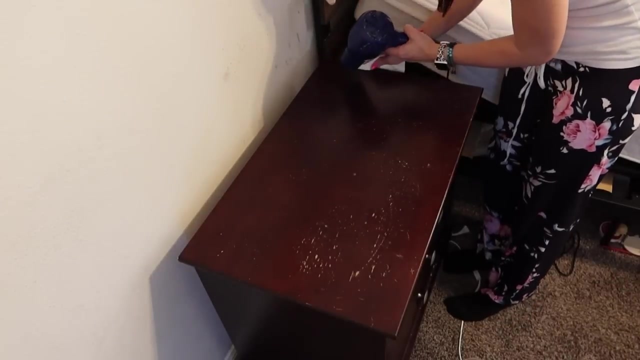 it right off. So we're going to give that a try. So I'm not sure, with this hack, if you are supposed to do it over the napkin or you know, do it directly onto whatever you're trying to get the wax off of. But I found that holding the blow. 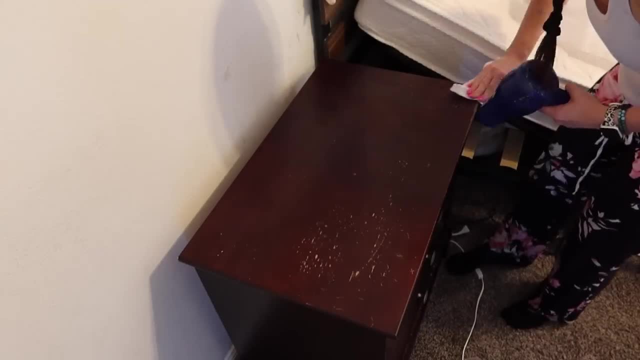 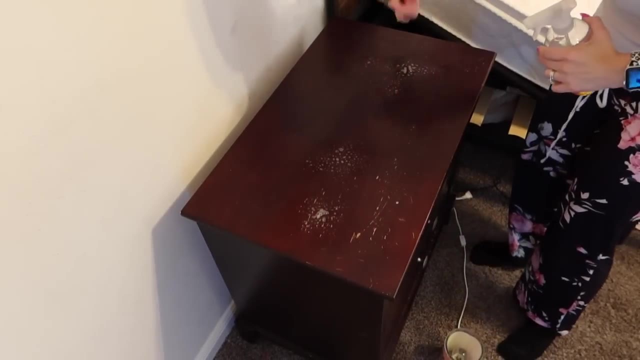 dryer directly on top of it would melt it a lot faster. And then I just wiped it quickly with the napkin and it did take it right off. So if you guys also have this problem anywhere, definitely give this a try. I'm going to show you how to do it. So I'm going to show you how to do it. I'm 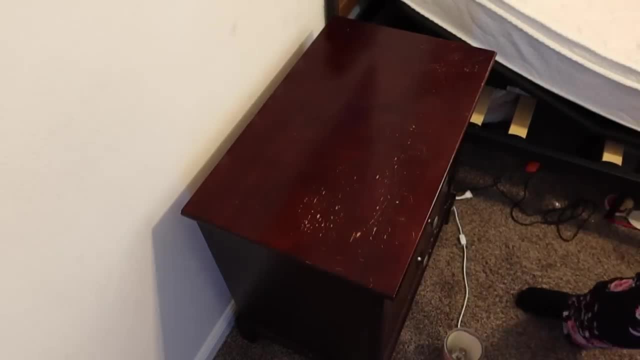 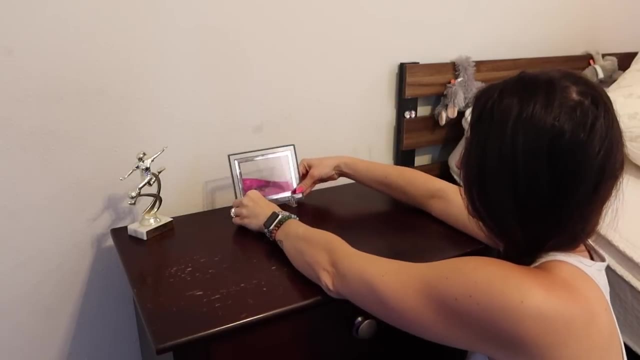 going to show you how to do it. I also tried it on the wall and it did a pretty good job at getting it off. But, like I told you guys, before we have flat paint, So it was no surprise that it didn't come completely off. I did, I thought I hit record, but apparently I didn't because I didn't have the 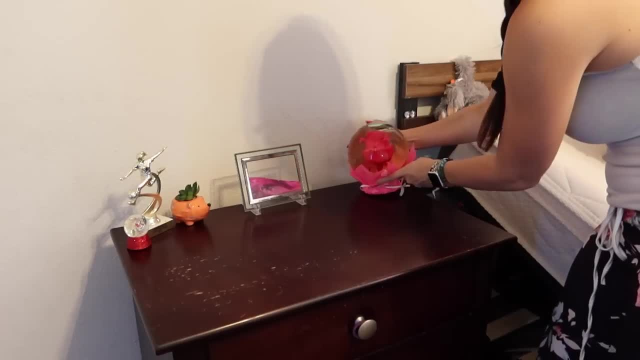 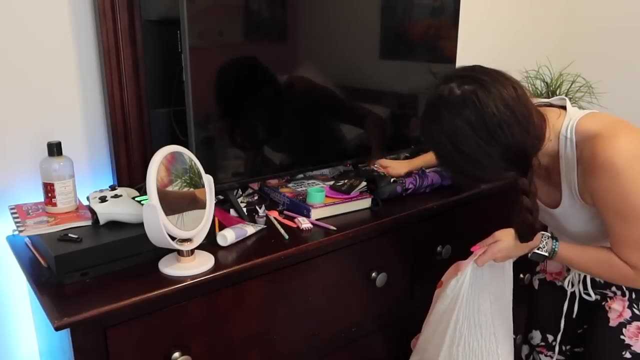 footage on here, but I did try it on the wall as well. I'm sure if you guys have satin paint it should come right off, because that's what I heard. But flat paint it definitely still left a little stain, but I'm really happy that at least it's not going to come off. So I'm going to show. 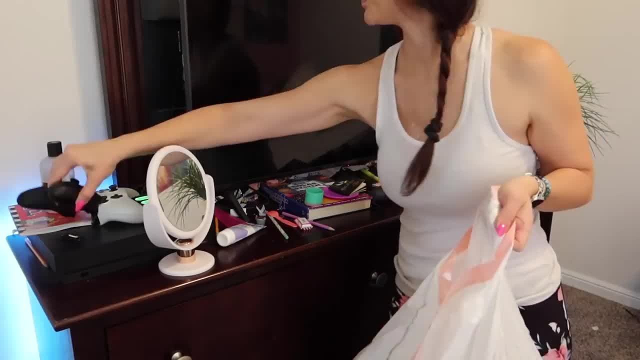 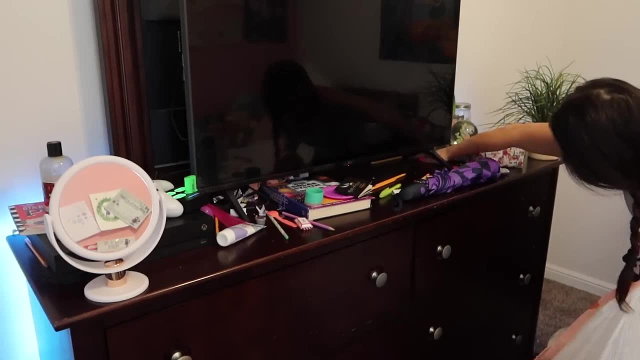 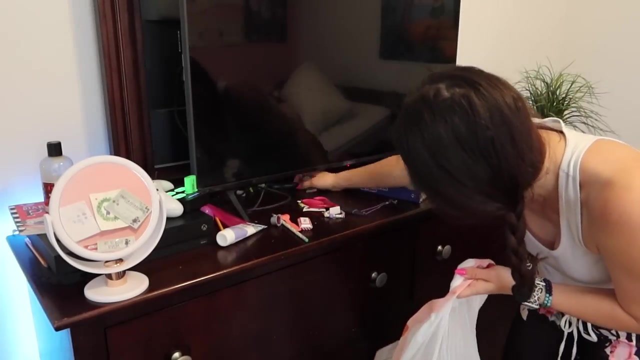 the nightstand is cleared off. I wiped it down with my wood cleaner and it looks so much better. but, yeah, no more wax in her bedroom because, yeah, that was not a very good idea. but now we're heading over to her dresser And, as you can see, she has so much trash up here. 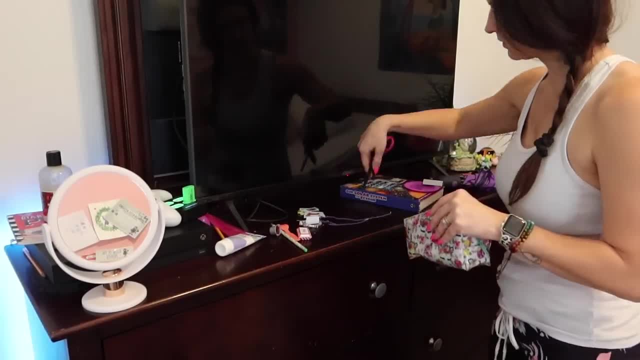 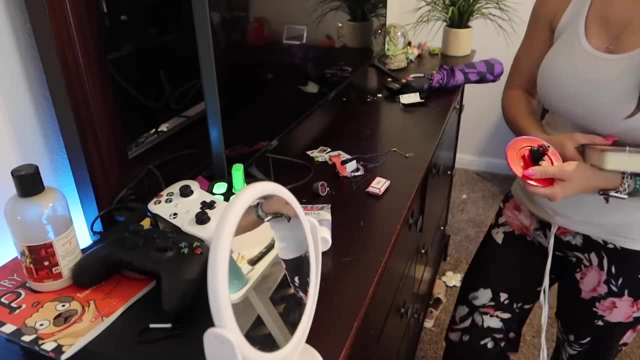 You guys, she loves making just like little arts and crafts things, So she often has tons of little cut up papers everywhere. So I'm just trying to get rid of all of the trash, clear it away for her. She actually loves when I clean her room. I feel like she gets. 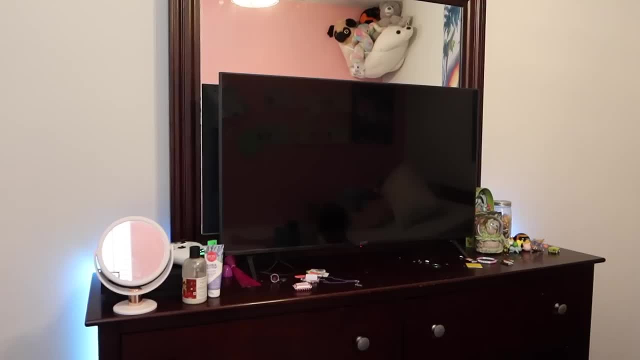 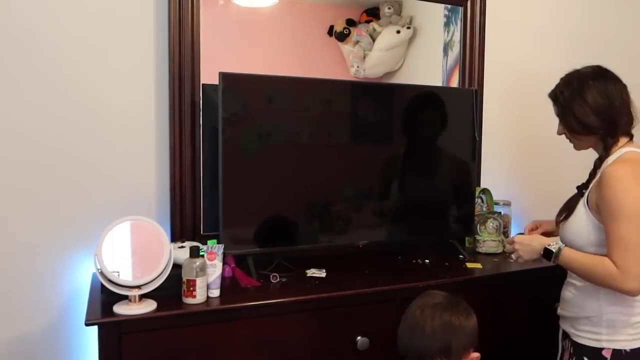 overwhelmed because she has so much in here which I do have. the rule every Friday they have to clean their bedroom before they can get on their electronics. But you know I told you guys this before. I don't like come in and do like a thorough check, I just open the door, make sure the floors 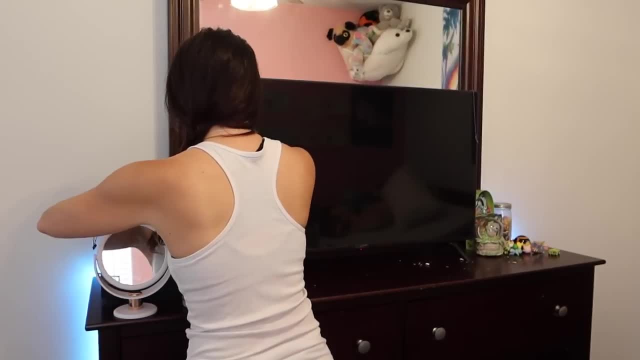 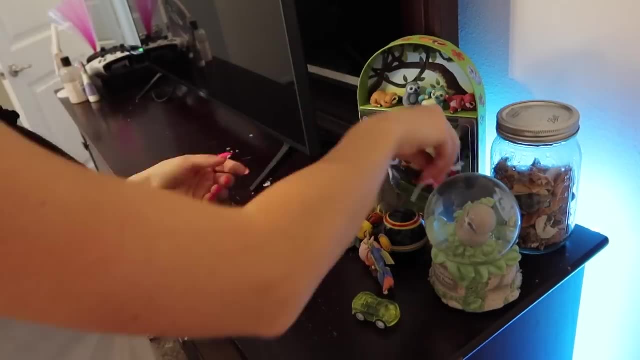 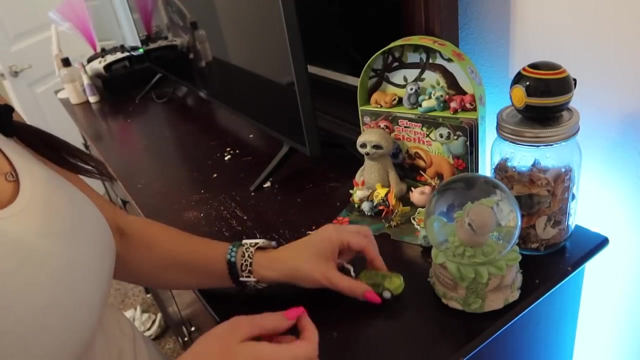 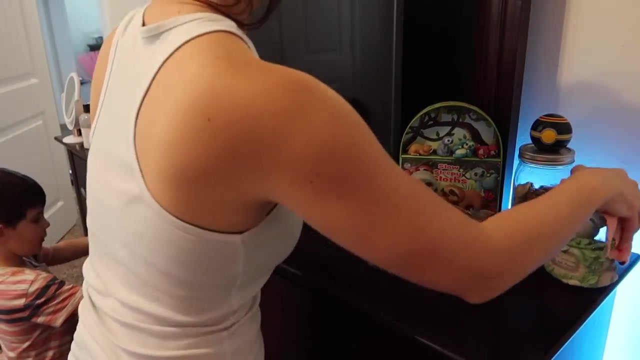 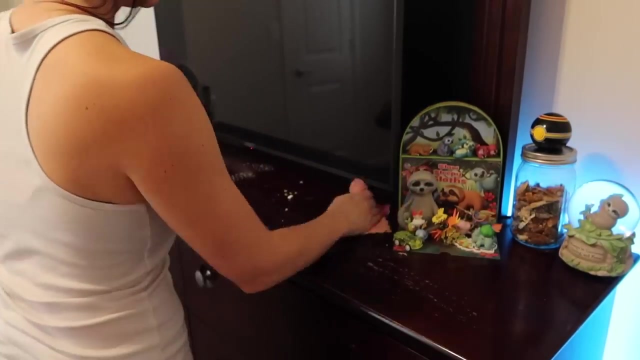 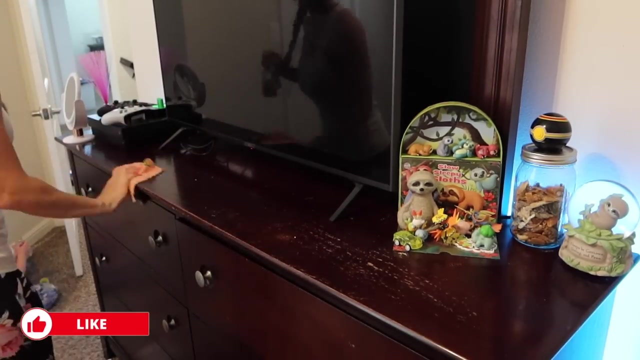 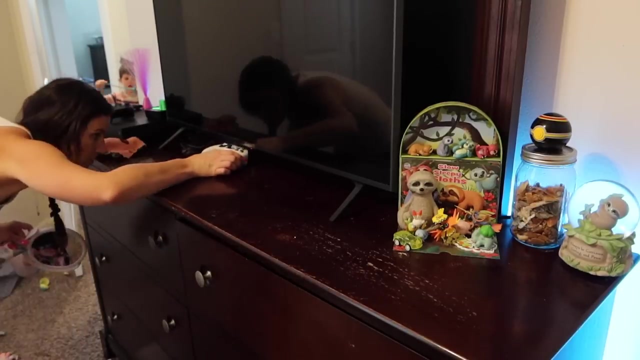 are clear and they can vacuum. So, um, yeah, every once in a while I need to come in here and give it a touch and do a deep clean. I thought I would take a moment to introduce myself, in case you're new here. I have been. 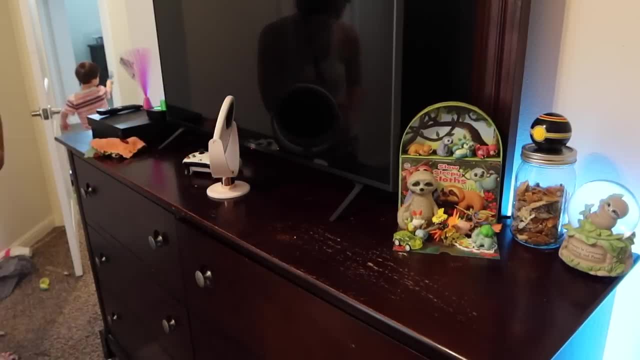 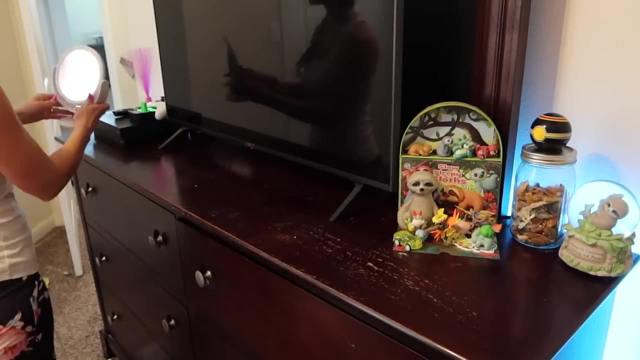 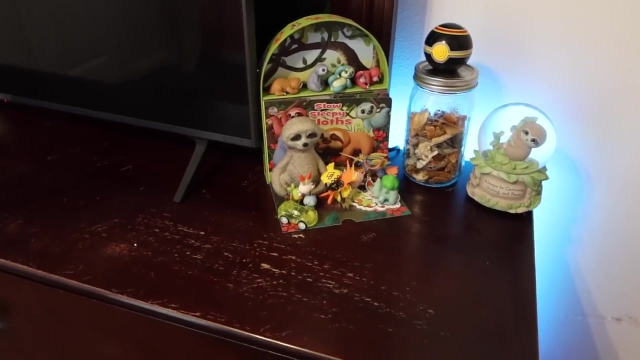 getting lots of new subscribers recently, So I thought I would just take a moment to tell you a little bit about myself. I am a stay at home mom to four. I have two girls and two boys, and their ages are 12 all the way down to three. So on my channel I love sharing realistic cleaning. 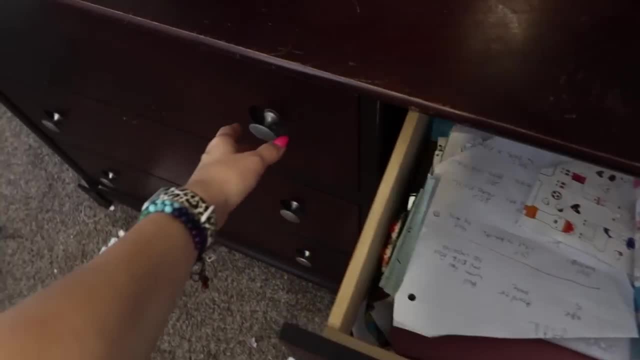 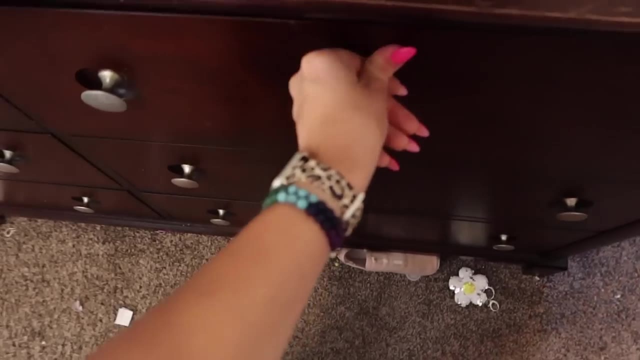 motivation, the everyday messes. I love sharing realistic cleaning motivation. I love sharing decluttering, organizing and I'm always showing you guys the real mess- Not no cookie cutter, Pinterest, mom style cleaning. This is like legit cleaning. This is what my house actually looks. 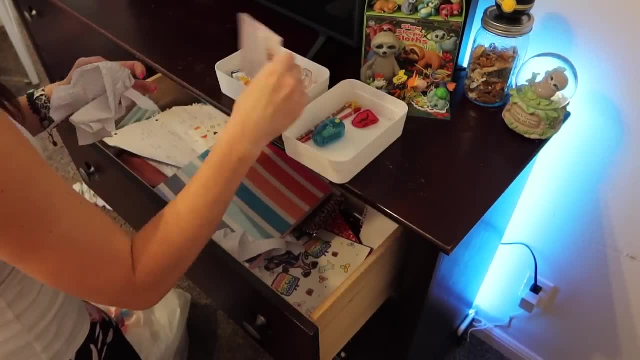 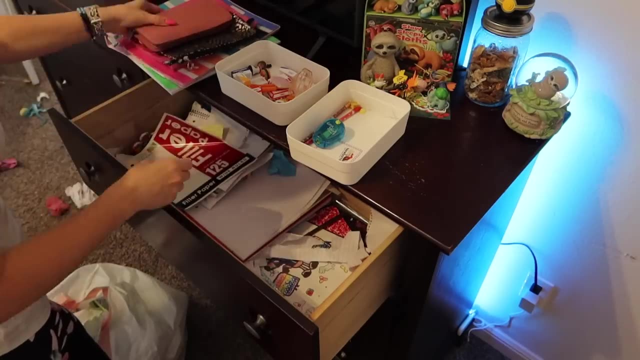 like We are not perfect. My house is not always clean And I really love sharing that because I feel like on the internet we often compare ourselves and feel like we're not doing enough or we should be doing better. But you guys. 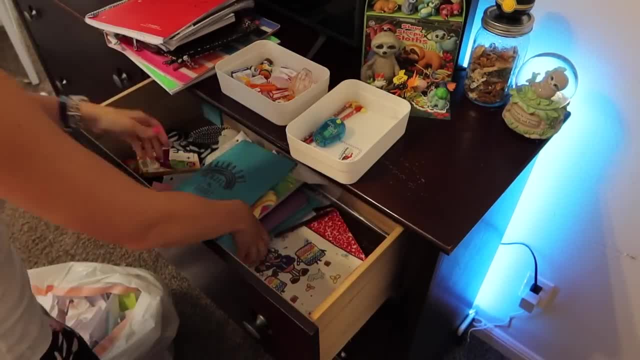 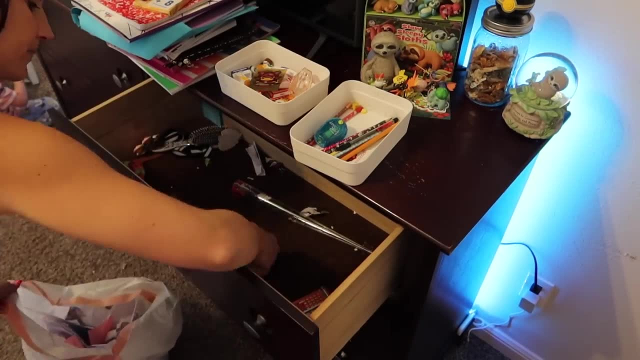 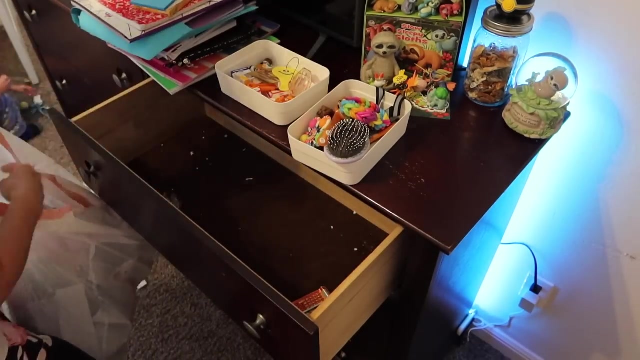 whenever I get done cleaning, as beautiful as it looks, it never lasts long. So I just want y'all to know that you should not expect your house to look perfectly clean all the time, because it's just not realistic. So I hope when you guys come to my channel you feel motivated to clean and you 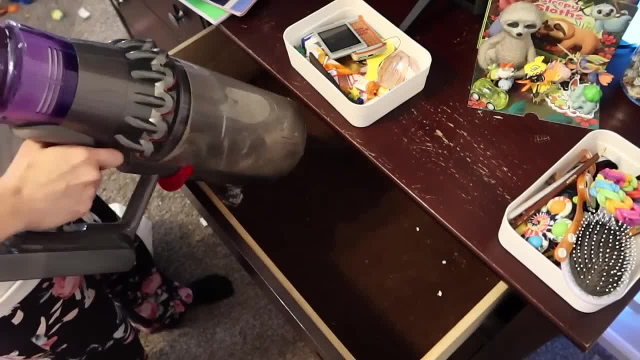 also feel like you can relate because your house looks exactly like mine. So that is what you're going to get on my channel. It's going to be a lot of fun. I hope you guys enjoy it. I hope you enjoy it. I hope you guys enjoy it. I hope you guys enjoy it. I hope you guys enjoy it. I hope you. 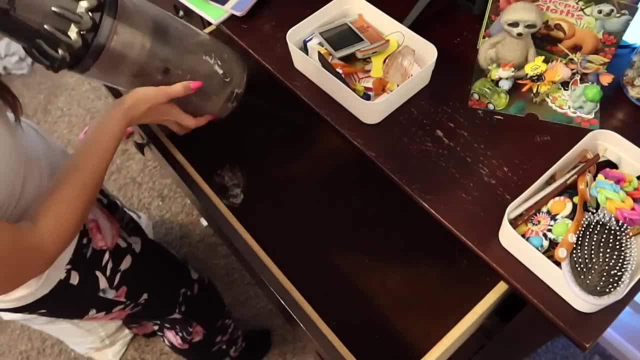 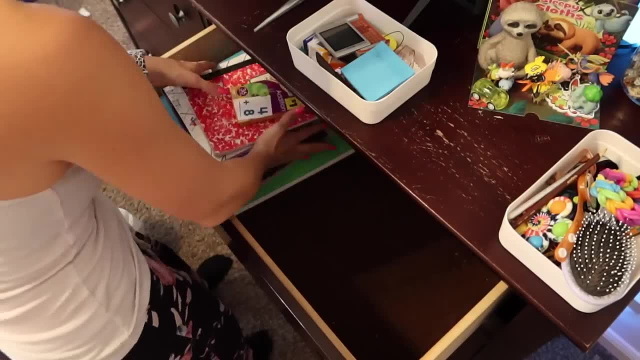 absorb it in your own right way. So this is the real deal, Mom, like cleaning. and as for me, I have been married for 14 years, almost 15 the summer to my high school sweetheart. we have been together so long. I can't believe it's almost been 15 years of marriage. 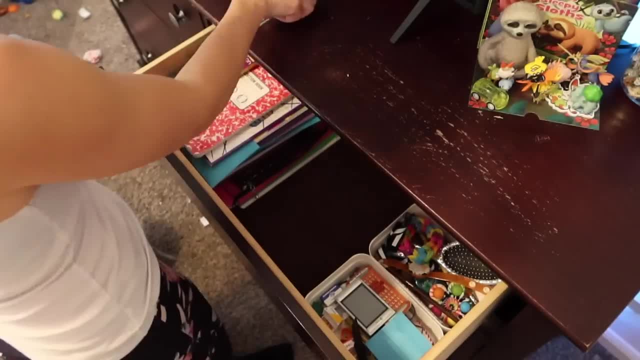 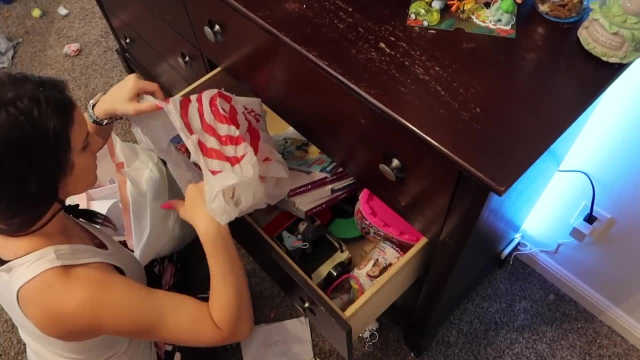 but we are originally from Virginia. We currently now live in West Texas And we really love it here in Texas. It is definitely a lot different than living on the beach. DOUGLAS boast Student Mishi Ajayi. Mishi Hai. heat Student Mishi Hai. 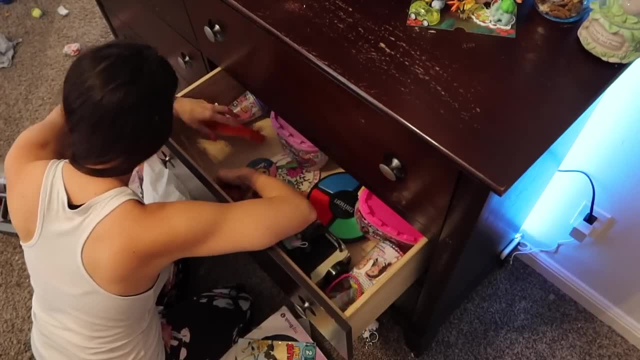 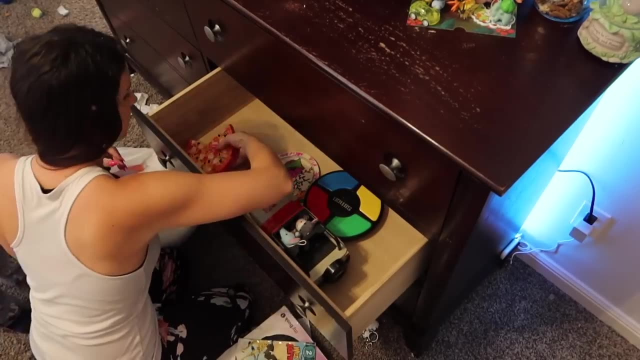 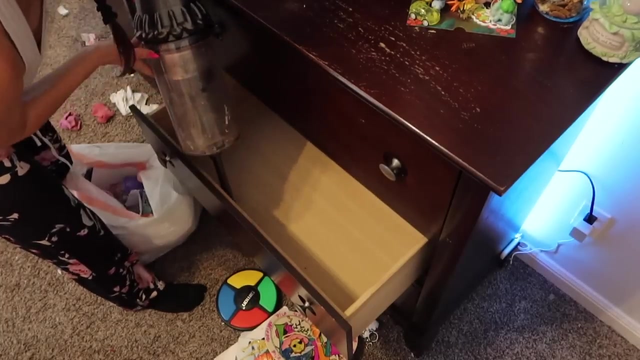 grown to love it over here. I am a huge fitness advocate. I love working out, I love weightlifting and learning about nutrition. That's like my jam. I love sharing about it on my vlogging channel. So if you guys are interested in seeing like my everyday life and my workouts and all that stuff, 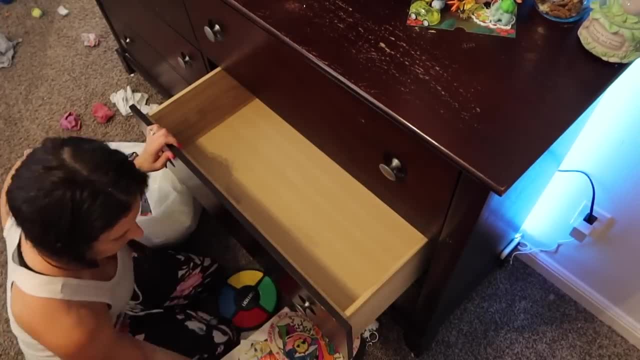 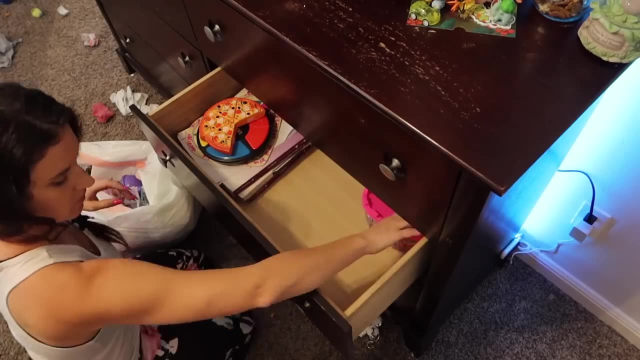 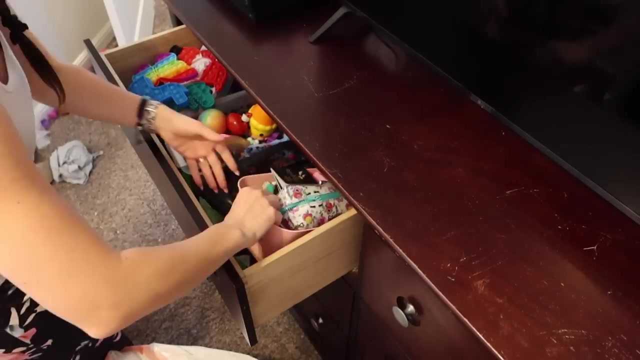 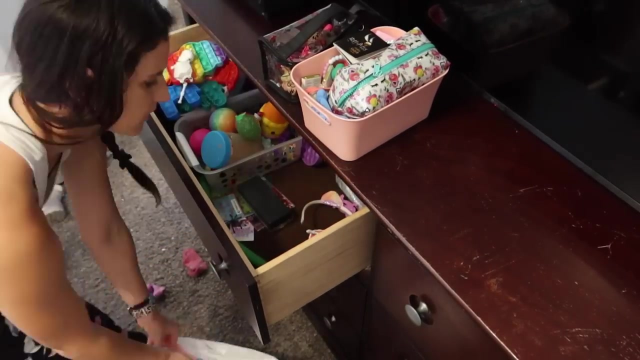 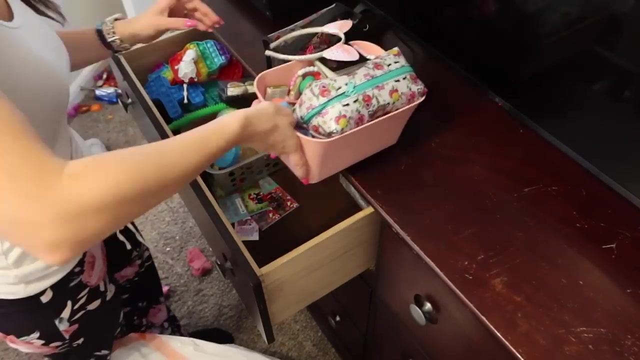 make sure y'all check out my vlogging channel, which is Ashley's Busy Life. I always have it tagged down in my description for you guys. This drawer was still fairly organized from the last time I did her dressers And we have these. 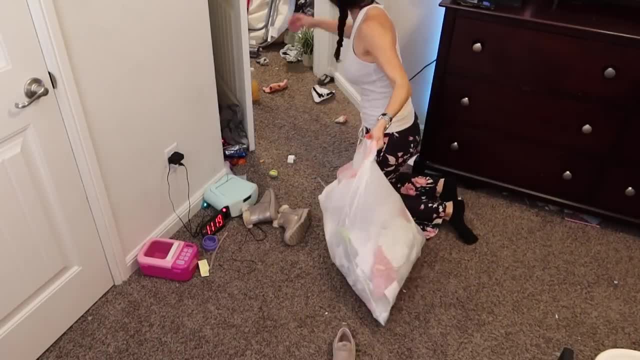 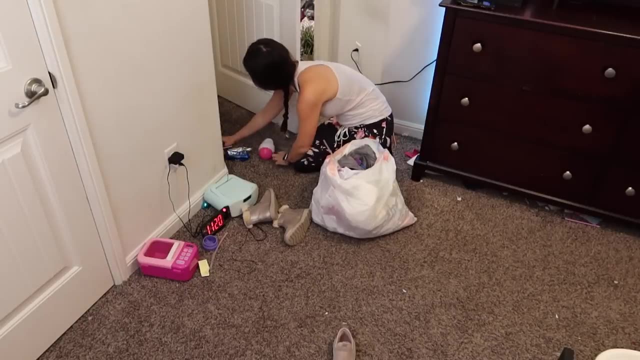 little Tupperware containers to you know, put your clothes in And I'm going to show you guys. store all of her fidgets. She loves fidgets. She doesn't really have too many toys but fidgets are definitely her thing, and mochis and all of that. So I just kind of straightened up a 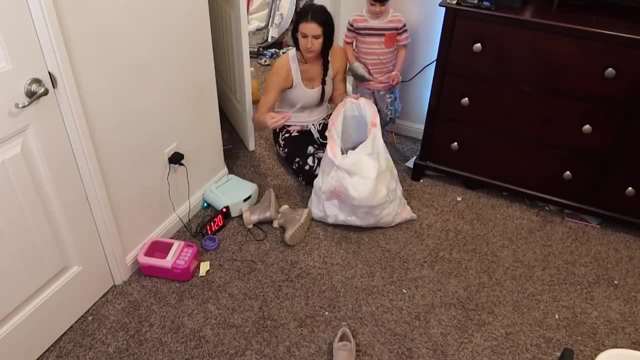 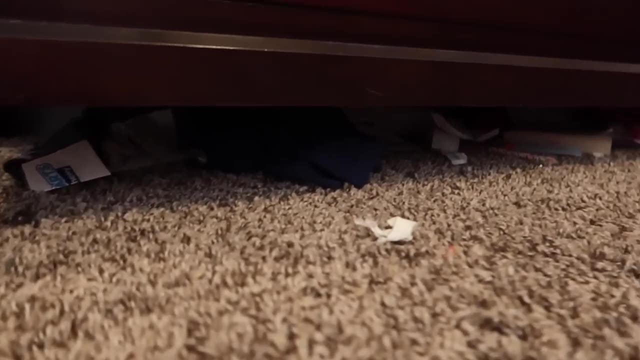 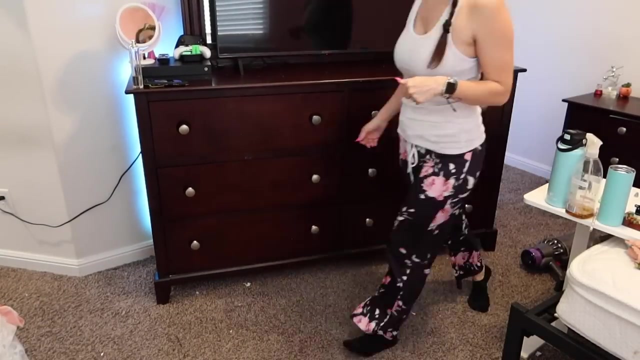 little bit in there, got rid of the trash and left it how it was, because those bins were just basically overflowing because she had so many, but they were still organized. So I left it as it was. but now it's time to pull the dresser out and see what we find underneath. here And boy. 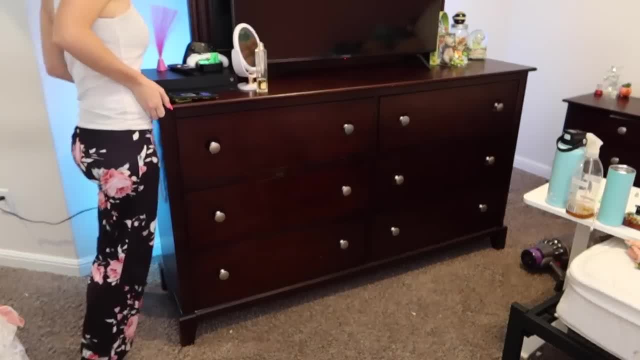 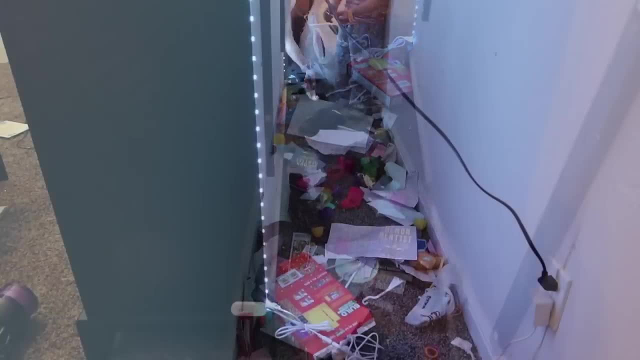 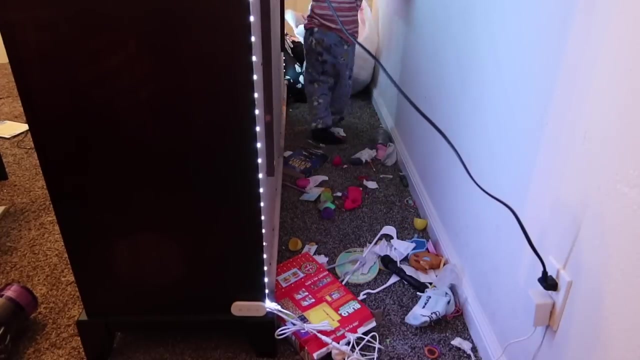 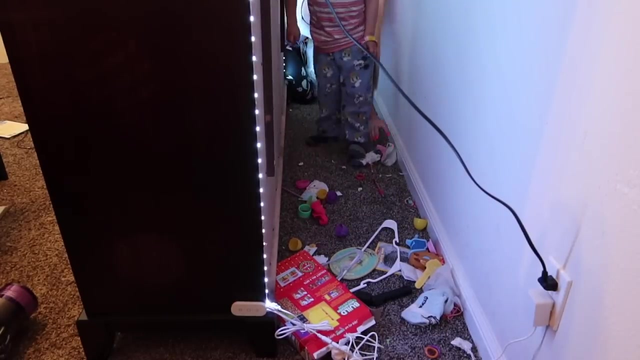 it's a lot. Ethan, my three-year-old, really wanted to help me clean behind here, So he got in there and helped me pick up all the trash. He has been so helpful recently, which is so sweet. Even whenever I'm telling the kids to like do their chores, he's always so quick to be like. 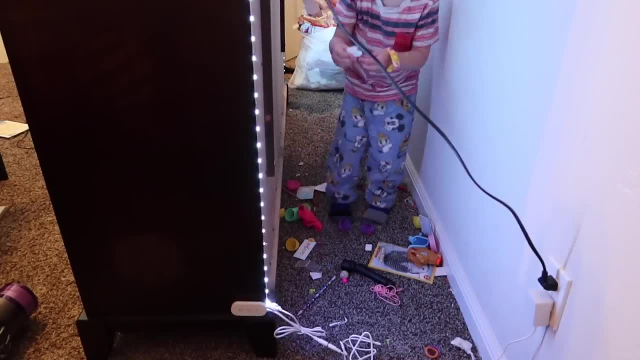 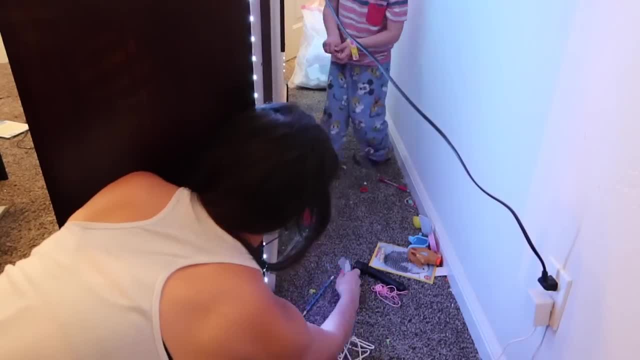 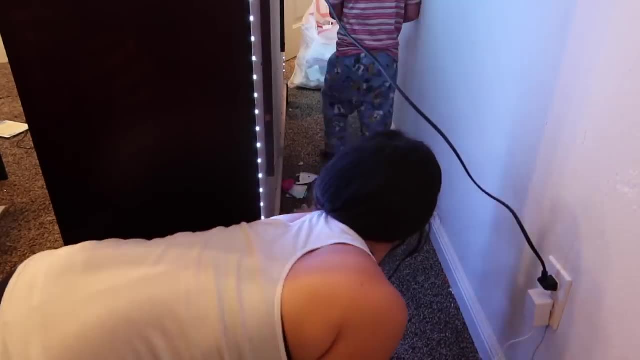 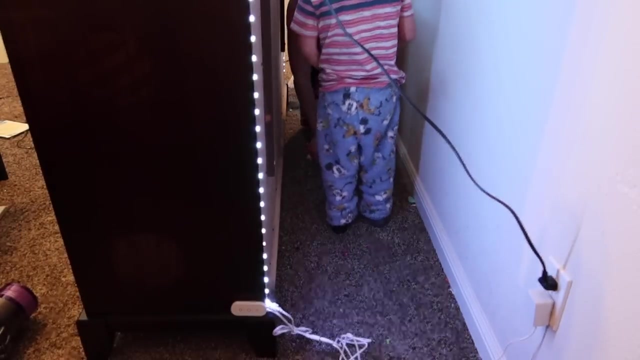 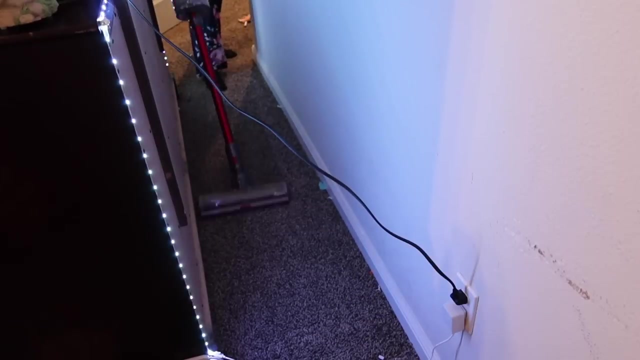 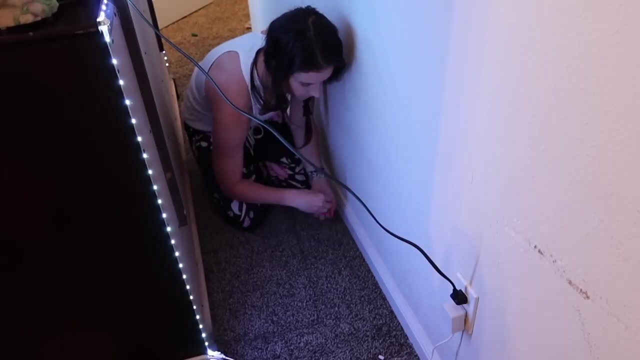 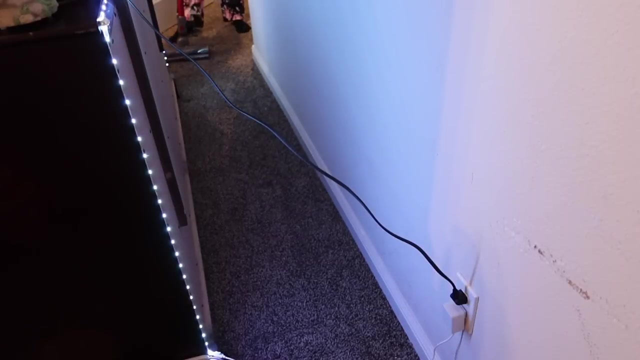 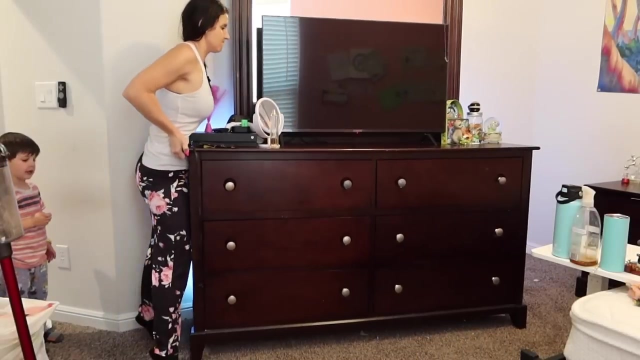 stays like that when he gets older, but at least for right now I'm definitely enjoying it. Keep saying I'll be fine, but how you know that I'll be there when it feels like I'm lying every time, I would love for y'all to leave me a comment letting me know if you guys are into like using 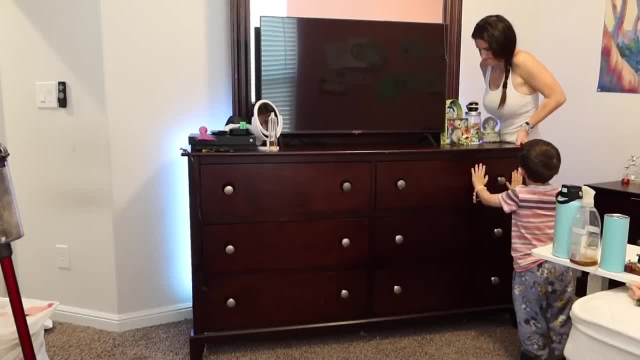 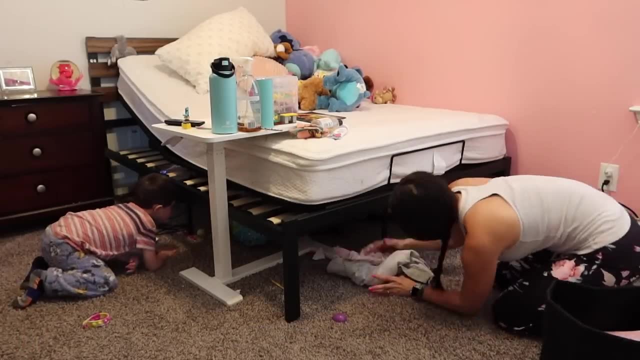 clean products that are more natural? or are you really not Picky on like what's in your cleaning products? You just kind of pick out whatever you, whatever you like, whatever smells good. I'd love to hear about it down in the comments. 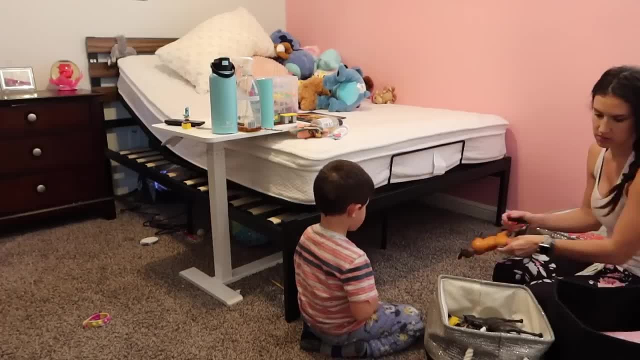 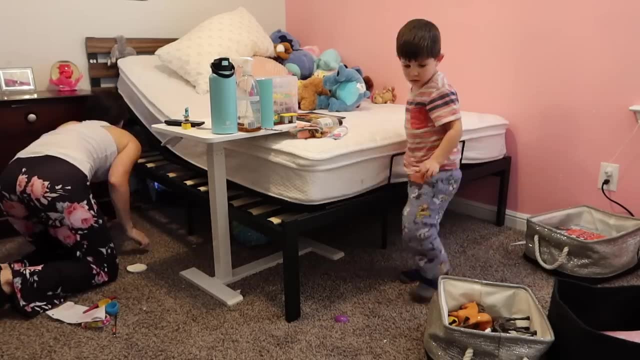 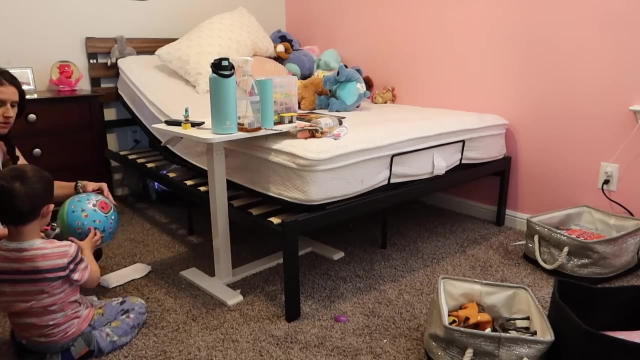 I typically just buy whatever I like and what smells good, But recently I have been doing tons of research into like different products and the stuff that's inside of them, especially like my makeup, my hair products, skin products, And I think I'm going to be doing a little bit of a 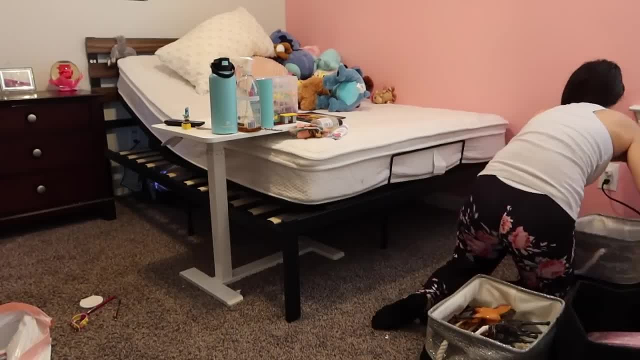 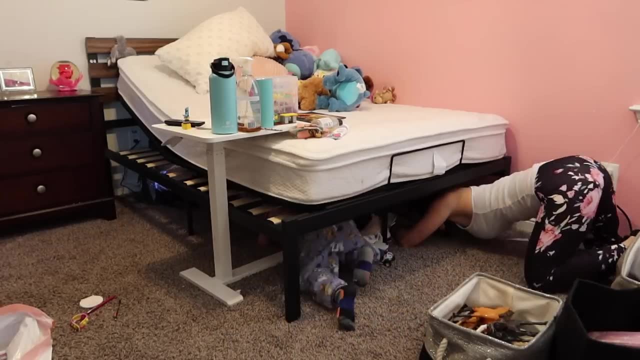 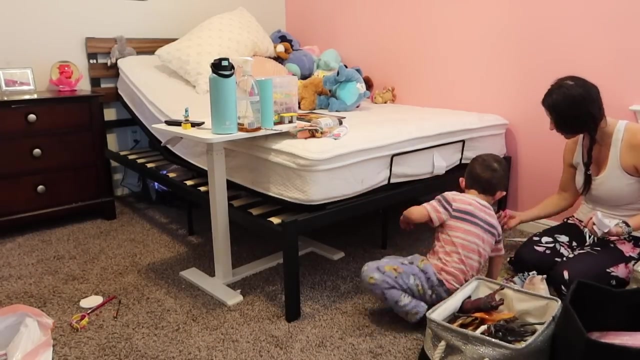 switch. I think I really want to start being a little bit more natural, especially on products that I wear every single day, like my makeup and my skincare, because obviously my body is soaking that up and using it every single day. So I feel like it's really important that I just make sure. 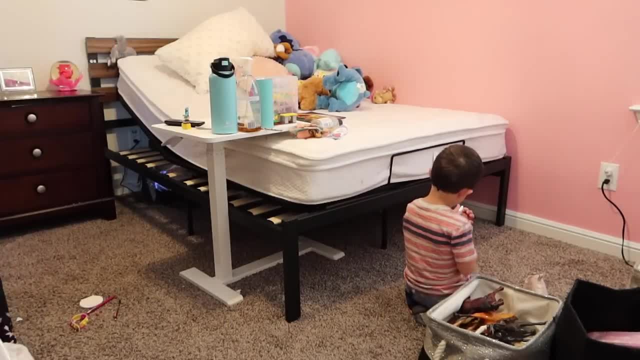 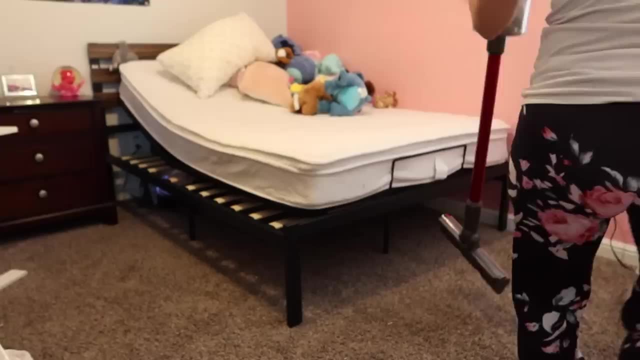 I'm not putting bad chemicals into me. So I am definitely starting to switch some products over and I'm kind of thinking about starting to look into the same thing For my cleaning products. I don't think I'm going to give up my pine saw, because I just use that on. 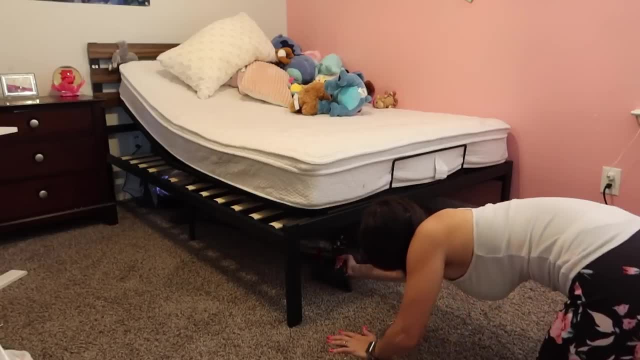 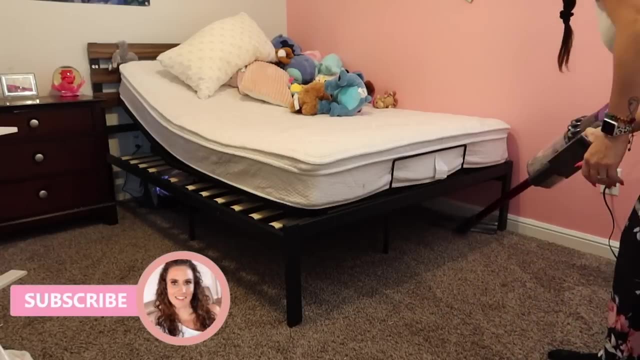 my floors, but I'm thinking like in the kitchen, where I definitely put like food on the counters and stuff. I think I want to start looking for a more all natural cleaner. So if you guys have some good suggestions that smell good- because y'all know I'm big on smell- I really like. 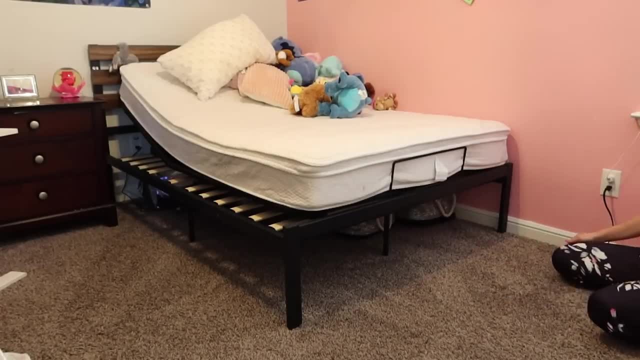 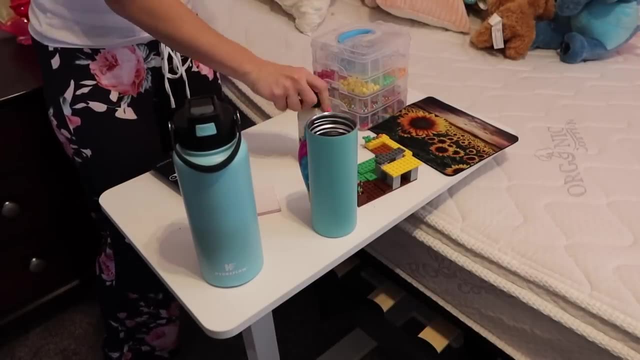 my house to smell like fresh and clean when I get done cleaning. So if y'all have a product that you're interested in, please let me know in the comments And I'll see you in the next video. Smells awesome And it's all. it's also natural. Let me know, Leave me a comment, because yeah, 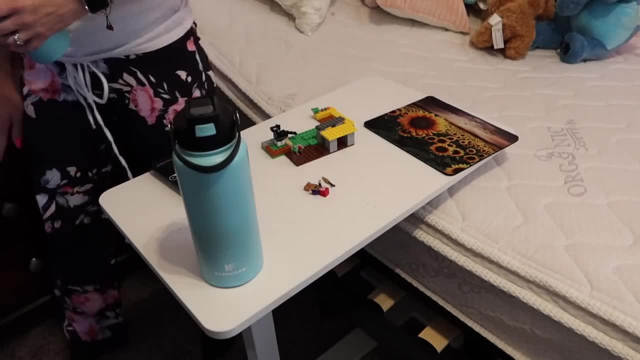 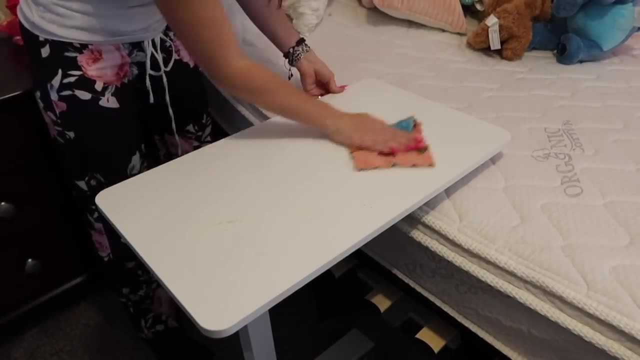 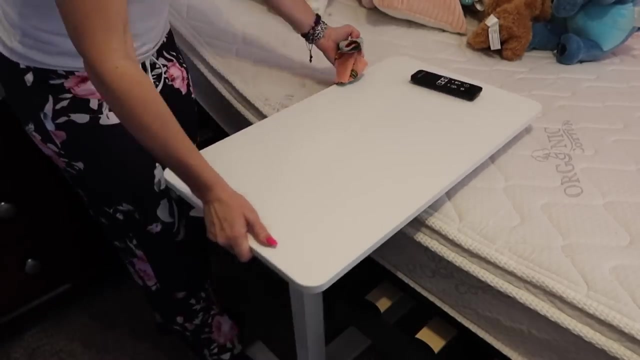 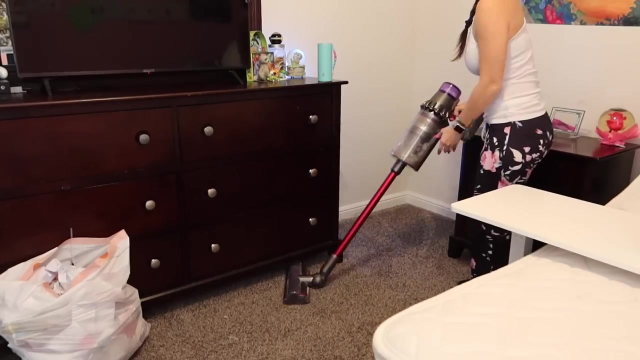 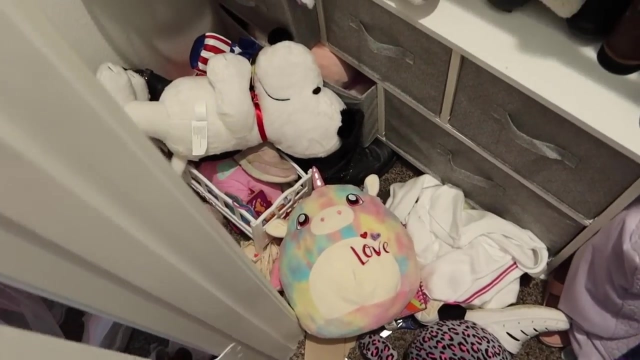 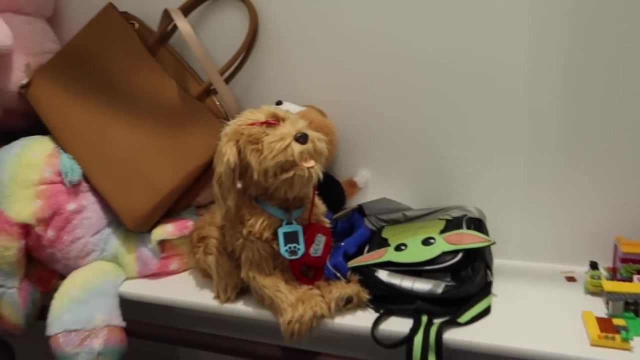 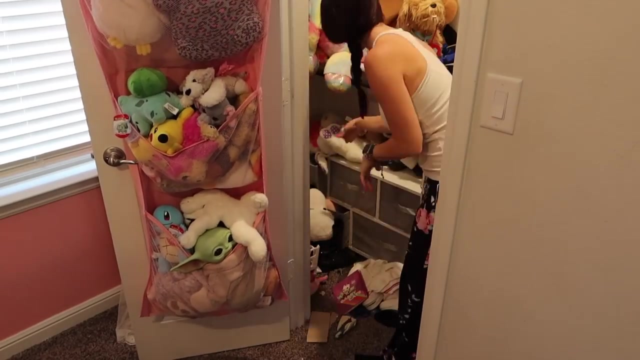 I really think I'm going to start paying more attention to the products that we're using Now. it's time to tackle this closet. It really wasn't terrible up on the shelves, but the floor was definitely cluttered. I was shocked at how much clothes I found in her bedroom. 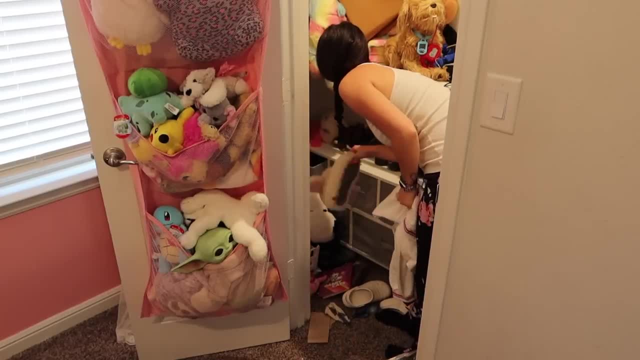 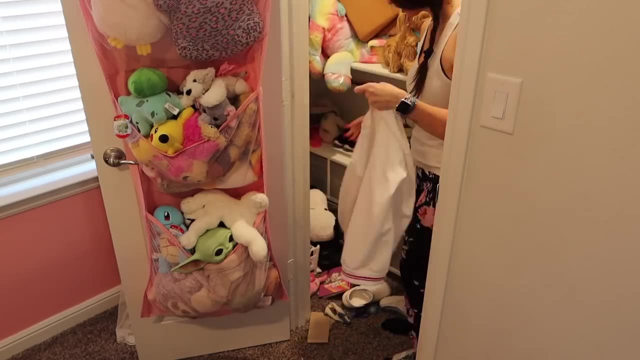 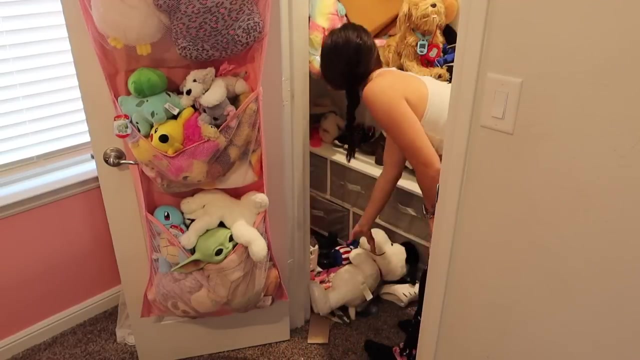 that was folded and clean and she didn't hang up. So literally that afternoon when the kids got out of school, I told them: look, this is the new rule. If I find any clean clothes in your room that is not hung up, you will be grounded, because I do not wash. 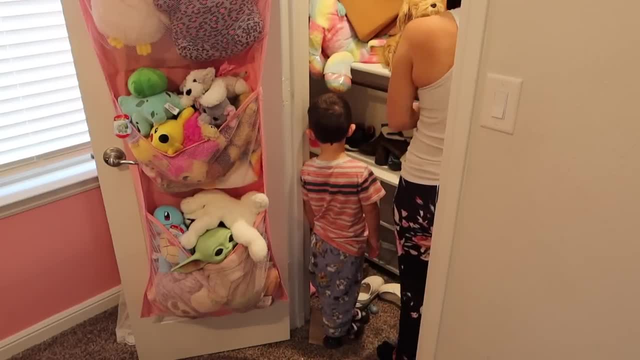 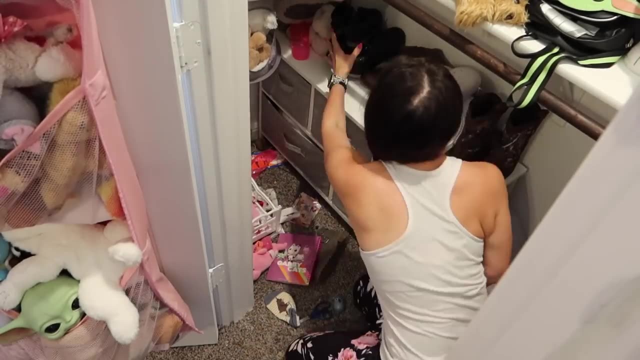 clothes and fold them for you to throw them in your room on the floor, Like, oh my goodness, you guys, I could not believe how much clean clothes- and it wasn't just in her room, It was in my oldest daughter's room as well. So yeah, new rule in the house. We are not doing that anymore. 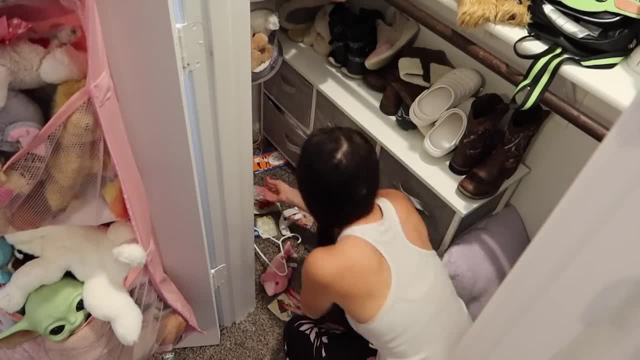 because we're going to have to do it again. So I'm going to have to do it again. So I'm going to have to do it again. So, yeah, the laundry is like my least favorite thing to do. So whenever I saw 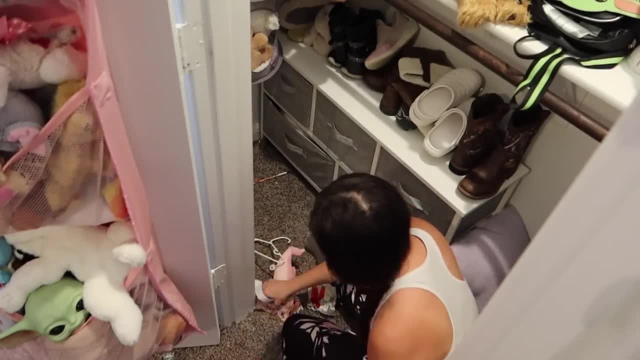 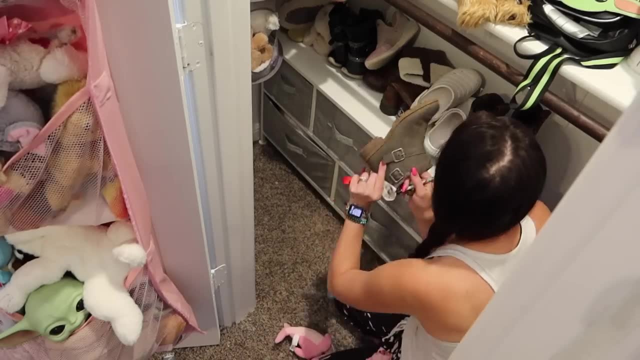 that I was like, oh my gosh, I could not believe that these girls- and you know, my boys- don't do it, because I still put away their clothes because they're still pretty little. But yeah, the girls are definitely old enough to not be throwing clean clothes on the floor. 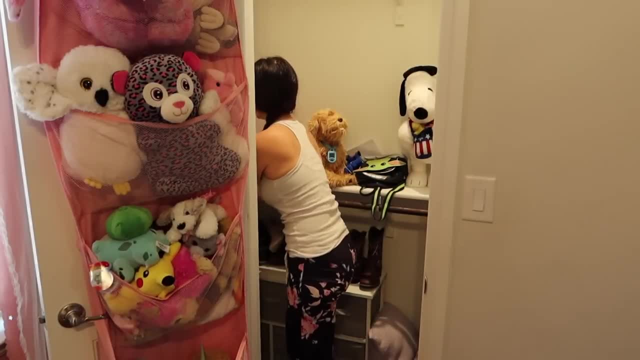 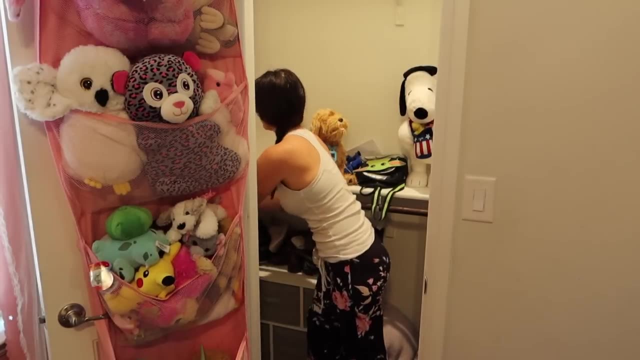 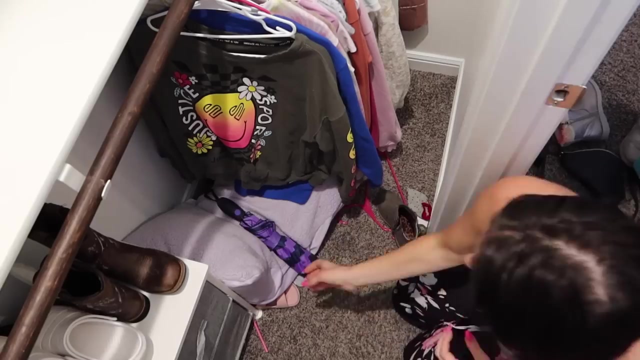 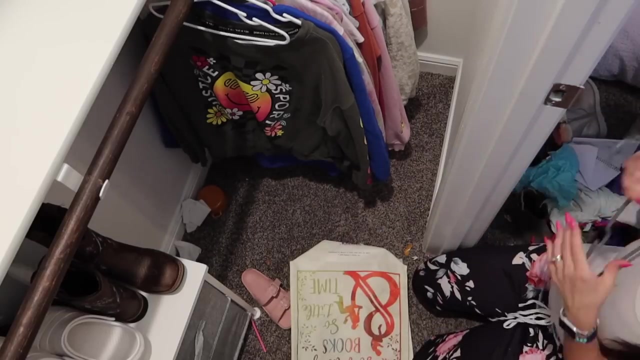 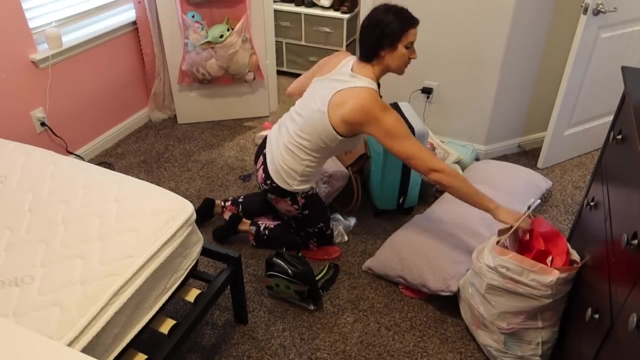 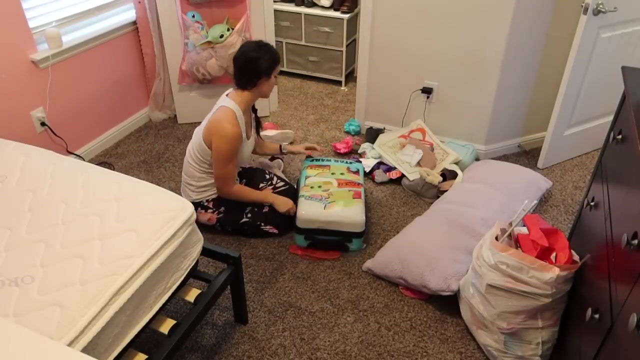 Let's go. So this was everything that was on the floor that needed to be put away. She had a lot of like purses and stuff, So what I like to do is store them inside of her suitcase. That way I can tuck them. 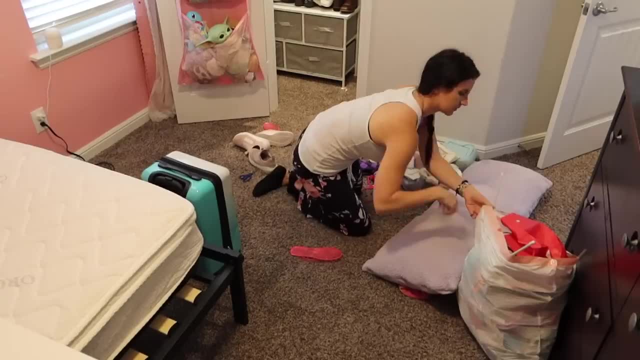 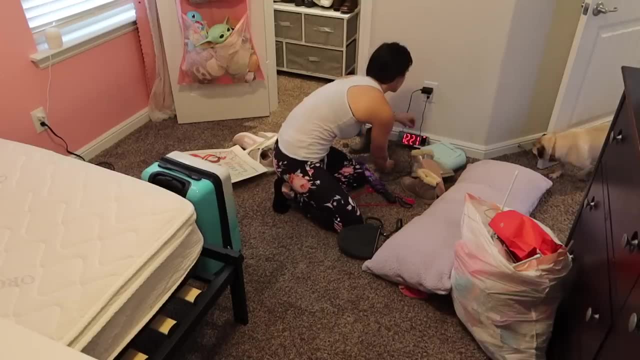 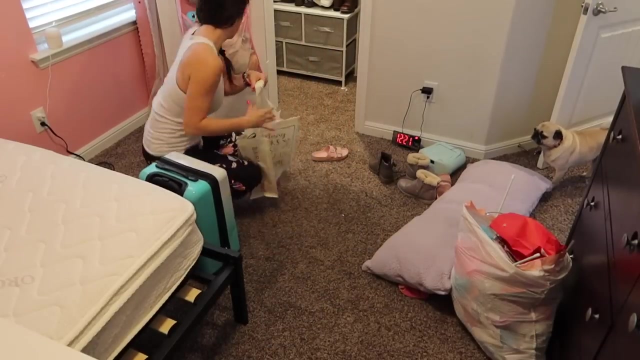 away Nice and neat. We really don't use the suitcase that often, So it's a great thing to store items in. Definitely recommend, if you guys have suitcases in y'all's closet, use it as storage. It's my favorite thing to do, but we're going to get this all put away. organize her shoes. 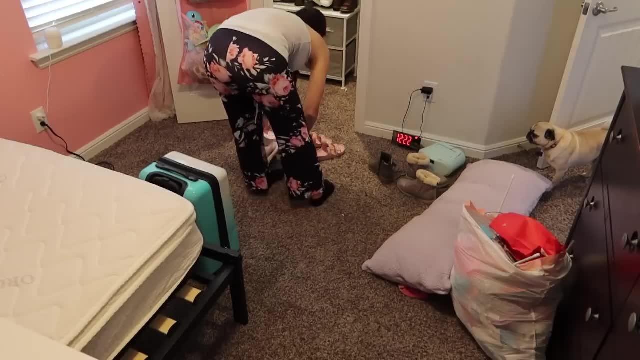 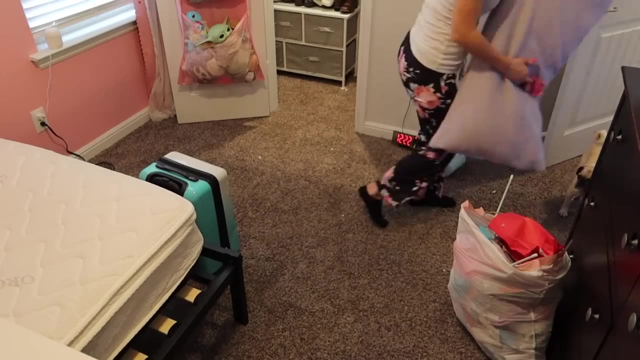 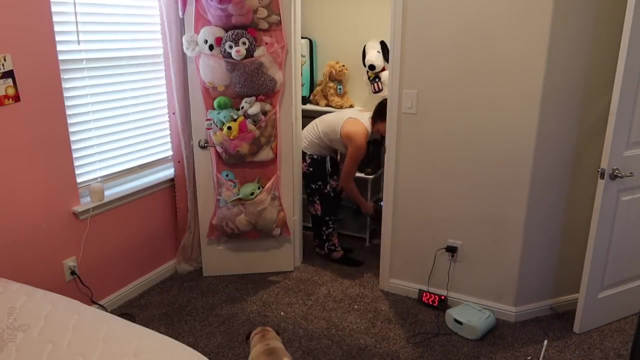 and then her room is finally going to be done. Just need to sanitize the doors, because you guys will see how disgusting they were. They were filthy. I mean. I have really been going through the entire house and cleaning walls and doors And I wanted to share something that one of my 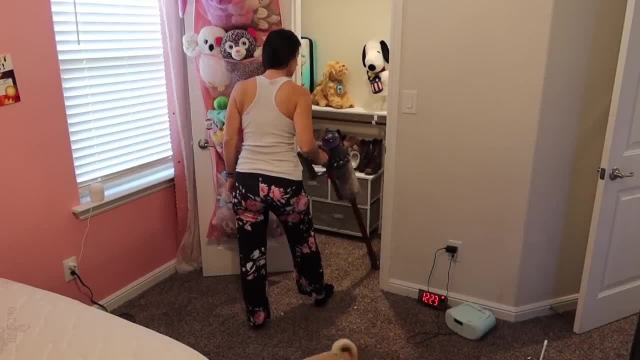 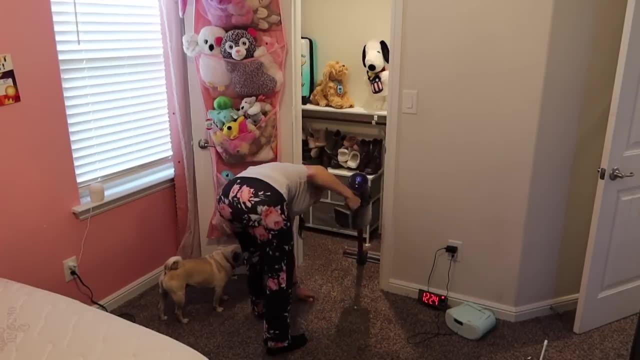 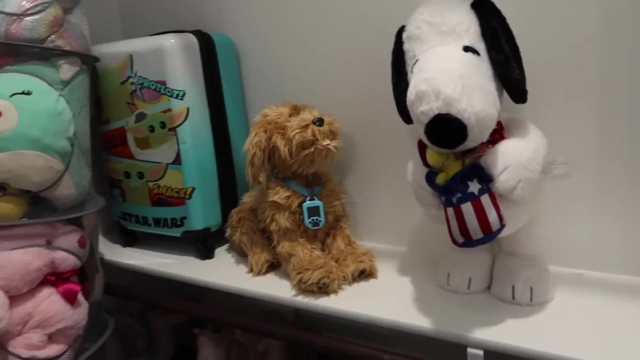 subscribers a comment that they left that I thought was so awesome And I haven't heard of this before. but she said that whenever her kids would get sick, she would actually steam the walls of the house and just walk around and steam all the areas to kill the germs, And I thought that 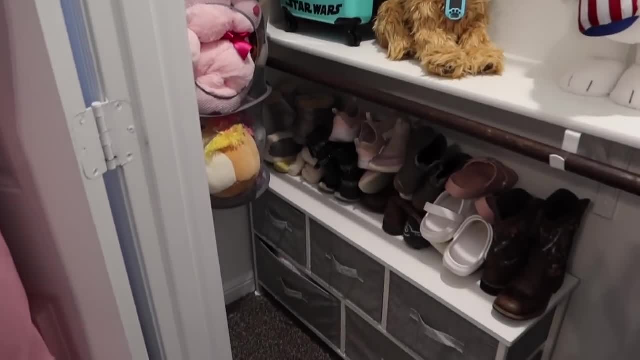 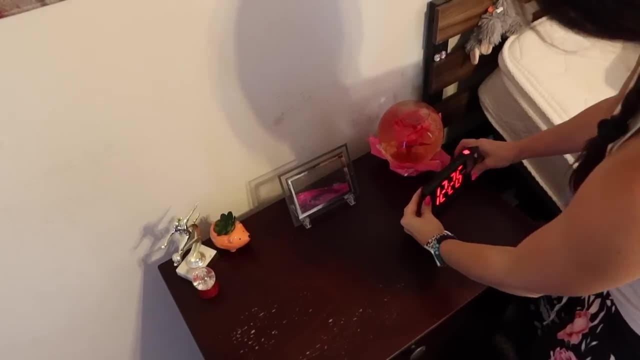 was such an awesome idea. I've never heard of that before. Let me know if that's like something you guys have done or you've heard about, but I haven't heard of it And I thought it was so genius because obviously it's going to kill germs, So just thought I would share it with all of y'all. 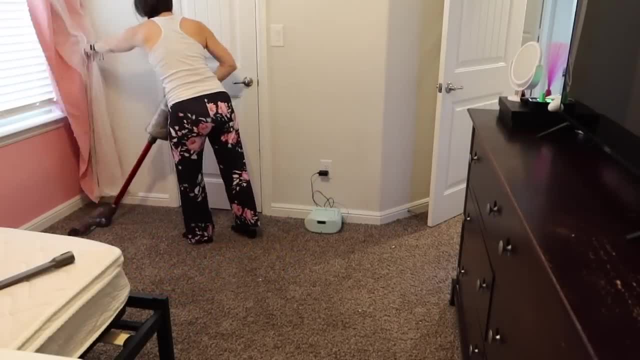 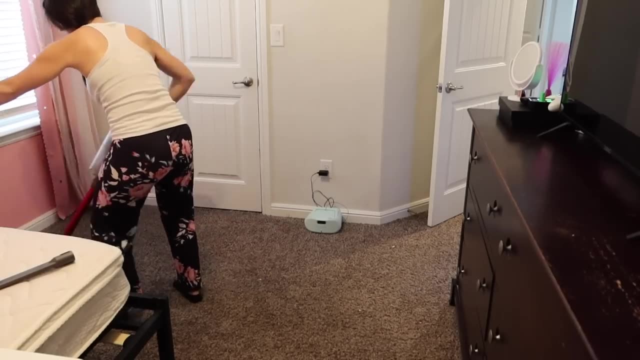 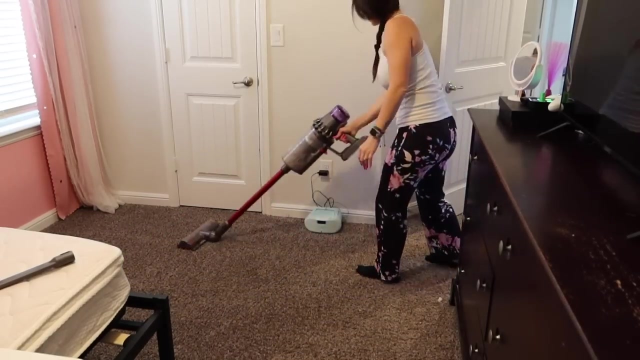 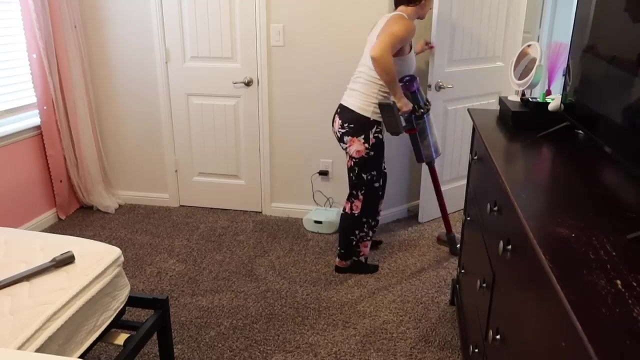 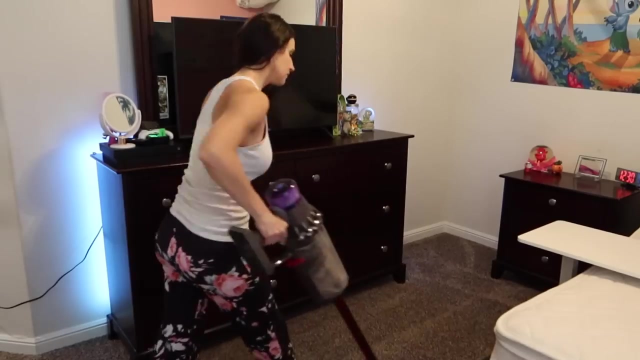 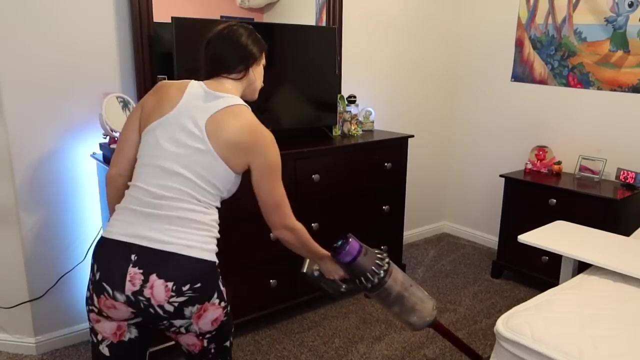 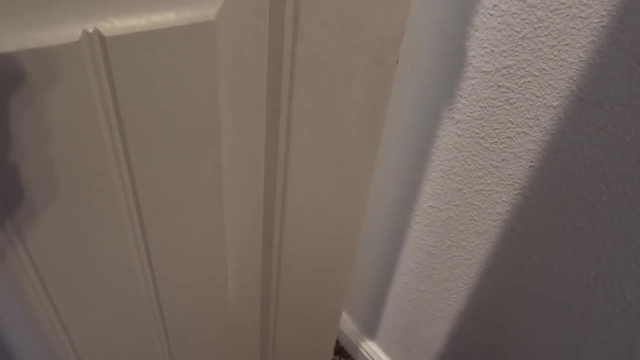 in case you want to give it a try the next time your kids are sick, because I'm definitely going to be doing this, because I do not want this stomach Bug in the house anymore- And I did not lie. Look how dirty the doors were. Oh my goodness, you guys. So we're going to be. 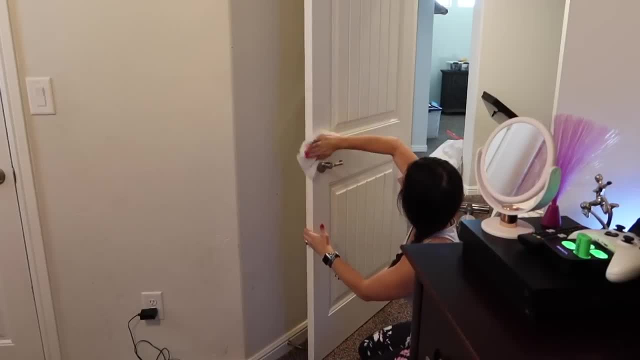 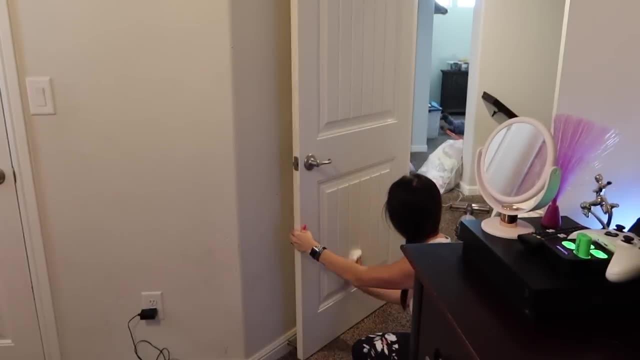 wiping these down with some antibacterial wipes to kill all of the germs. If the doors aren't that bad, I'll just use my wood cleaner. But since we had sickness in the house and they were so gross, I wanted to make sure I sanitized, And I'm going to be wiping down the light switches as well. 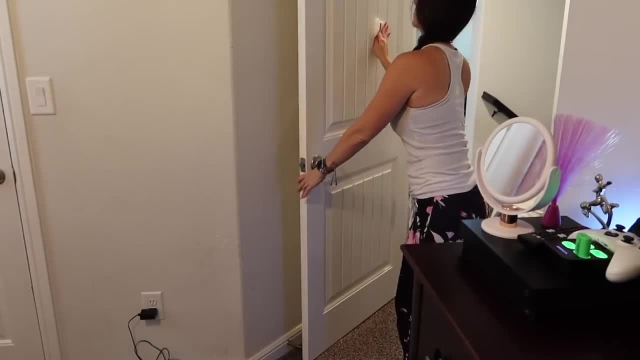 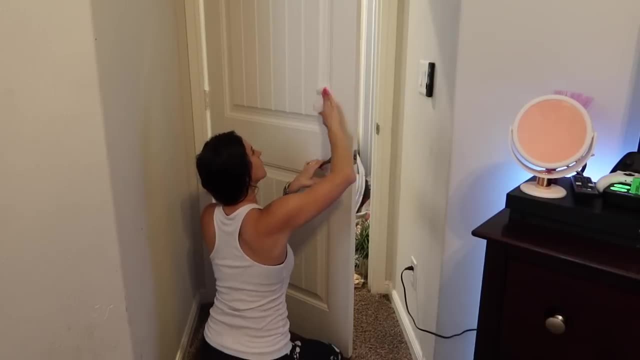 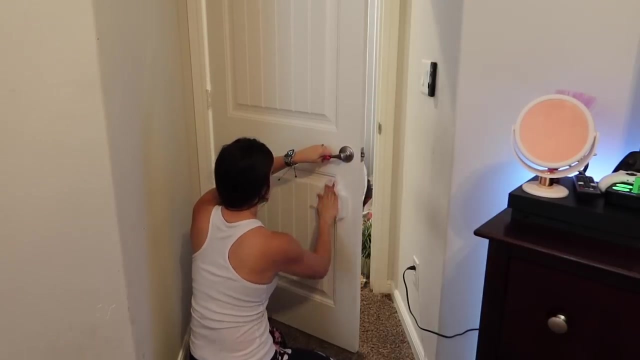 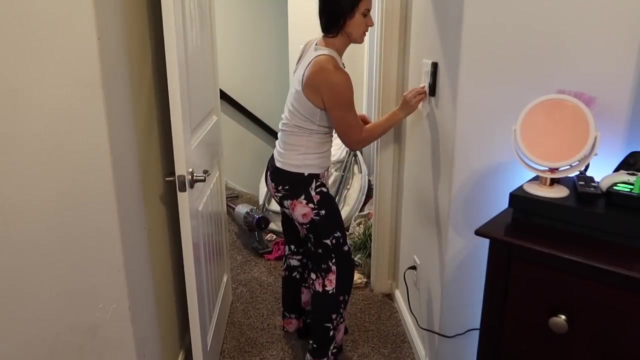 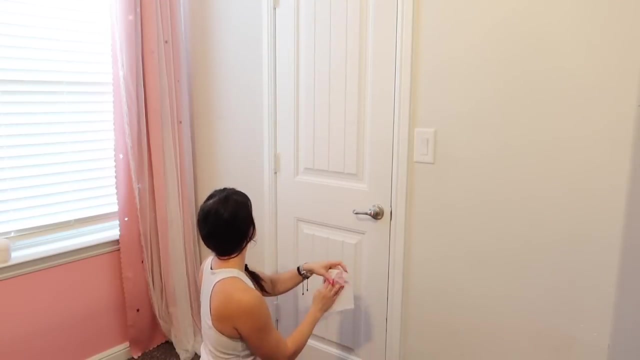 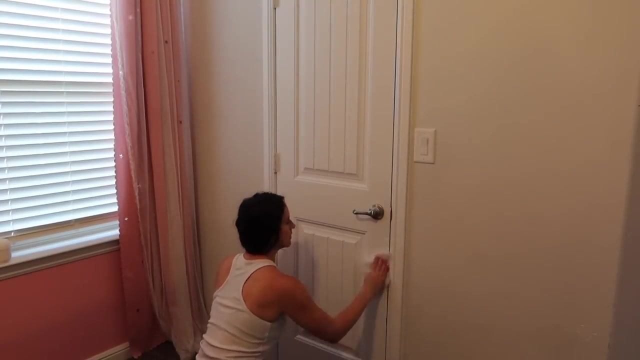 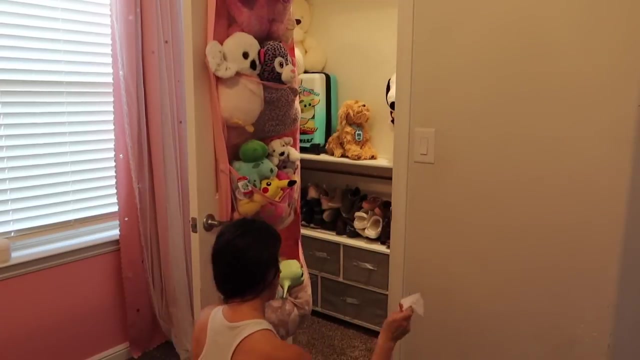 because they were also really dirty. So the Swamped out. So we're going to go ahead and I'm going to run through the doors and see if I can see any other things. This is a fleece, so you don't have to be wearing ones. 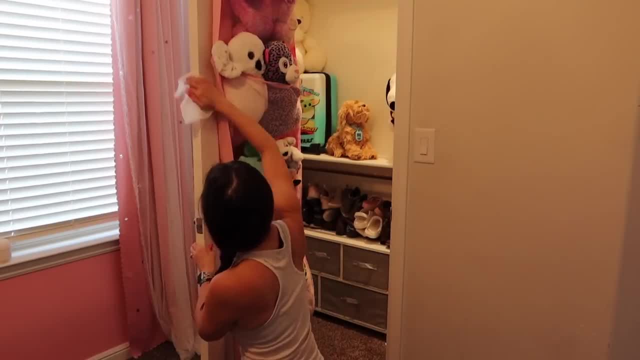 I'm going to walk you through the door now. Let's see They don't have the Braun leather. I don't know if you guys have seen the Braun leather. Okay, we're going to do the door area now. I'm going to go ahead and just fill the door and see that's clean. 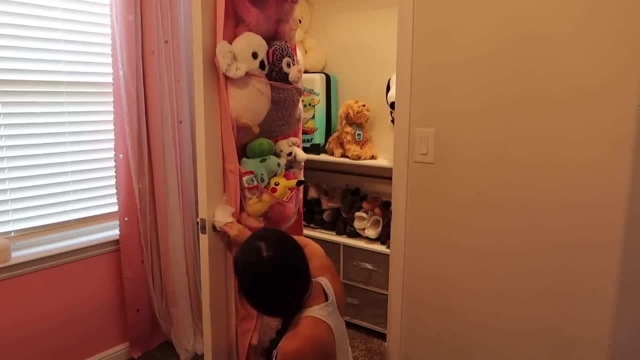 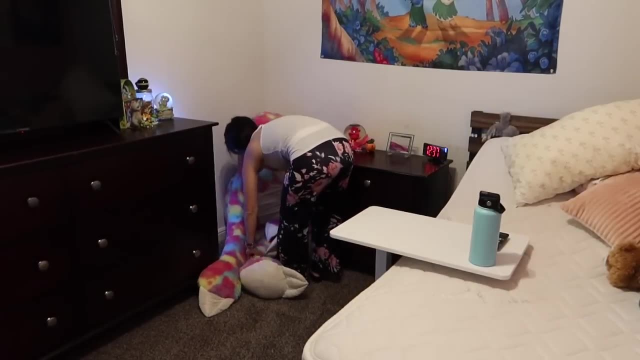 Now I want to be there and baby Now. Now it was time to put the last couple of items back into her room. Okay, to get her to get rid of this huge sloth for years now, but she loves it so much, so we just 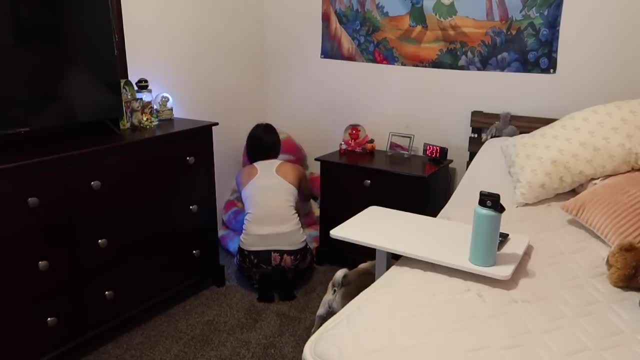 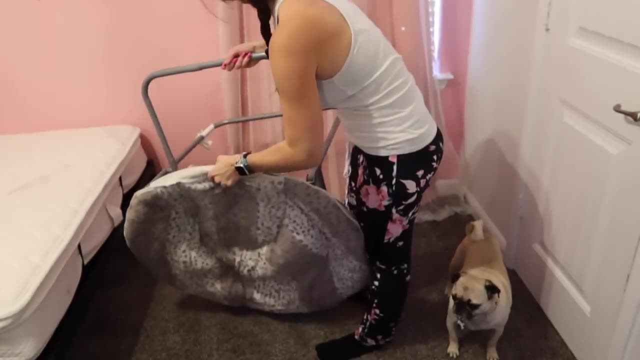 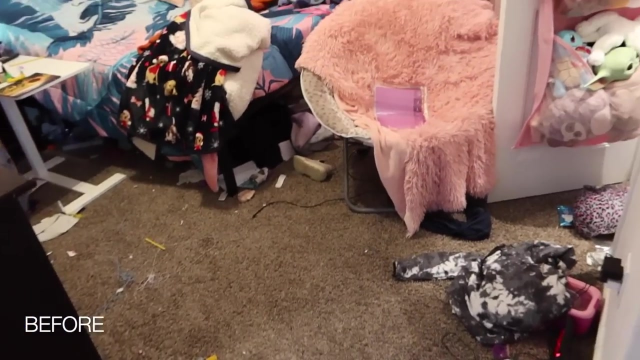 put it in the corner and she actually likes to use it as a little spot to sit in and read and hang out. so she still has it. at least it looks a little bit better in here now that we have all of her little stuffed animals, nice and organized and off of the floor and majority of them off of the bed. 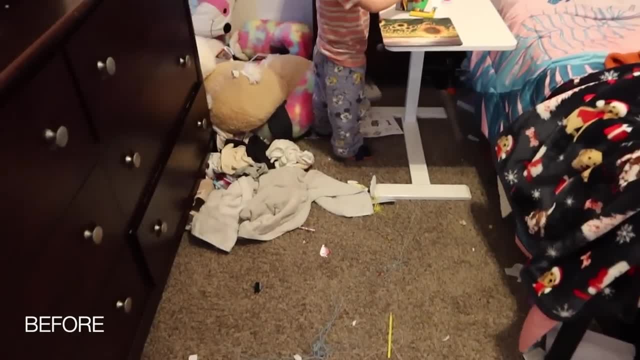 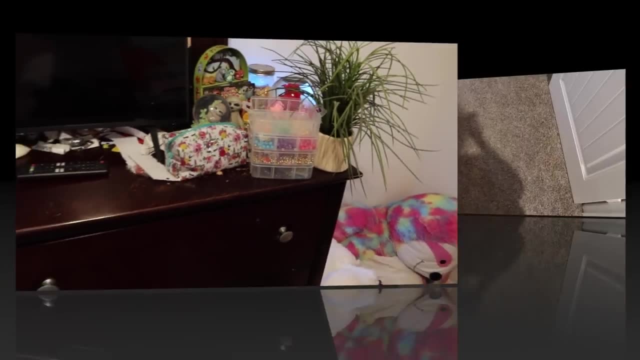 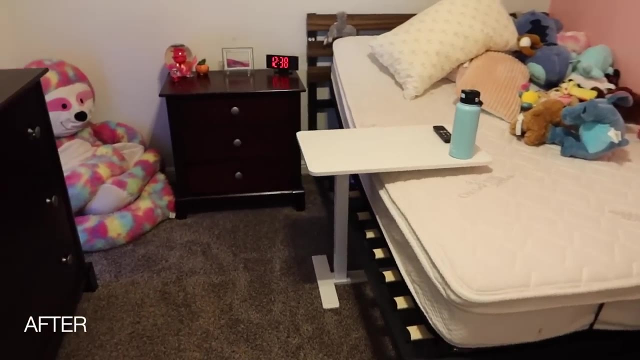 but before we do the reveal, of course we have to do the before so you can remember what it looked like. and then, oh my goodness, you guys, this is seriously the best feeling ever. every time i get done doing her room, i just feel the biggest sense of satisfaction. 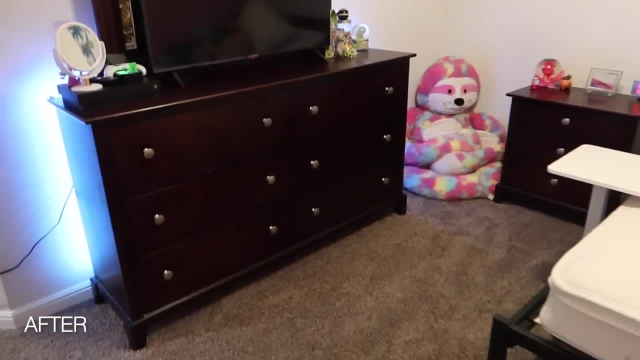 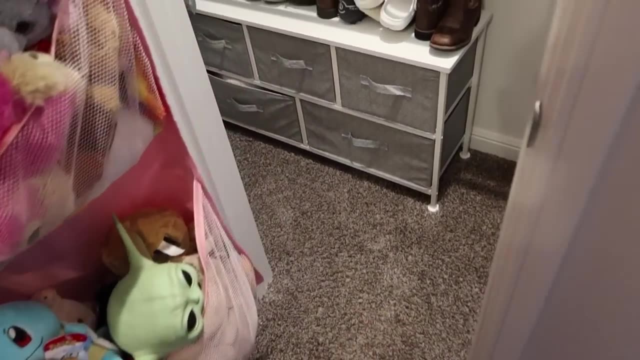 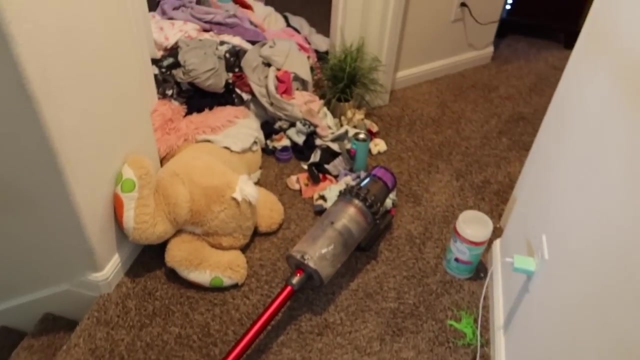 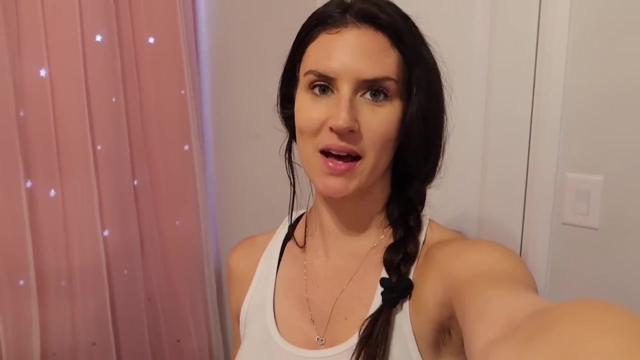 it just ah, it makes my heart so happy. i love doing deep cleans like this. so there's the entire bag of trash that i got out of her room and all of the laundry. oh, my goodness, my goodness, you guys. it feels so good to have this room spotless. i hope you all enjoyed this. 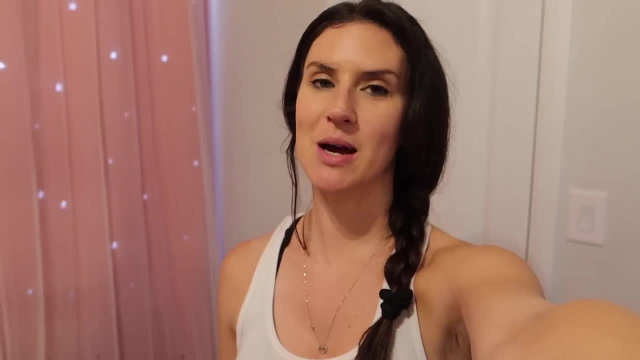 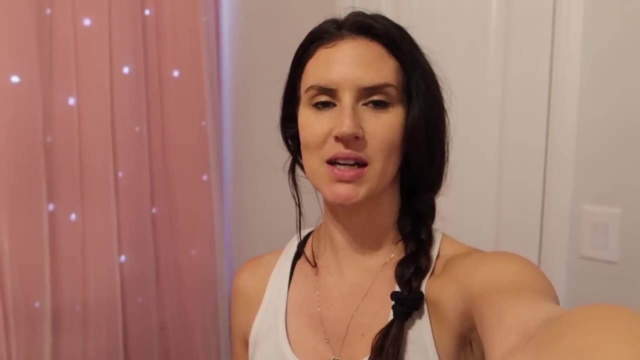 one. if you did, don't forget to give it a big thumbs up. it really helps out my channel. if you're new, i would love for you to subscribe. i upload cleaning motivation weekly and i would love to have you here. but i hope you all have a wonderful day and i can't wait to see you in the